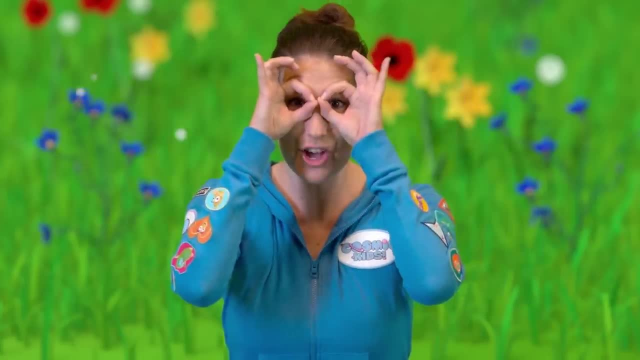 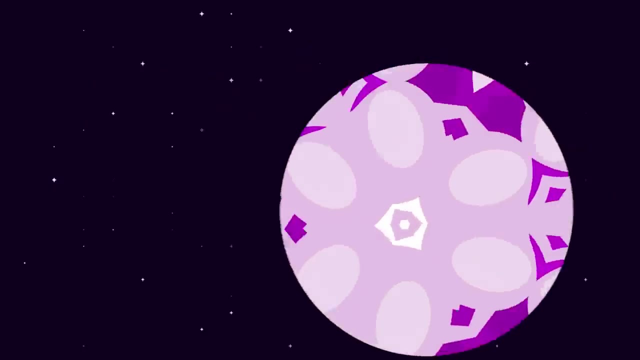 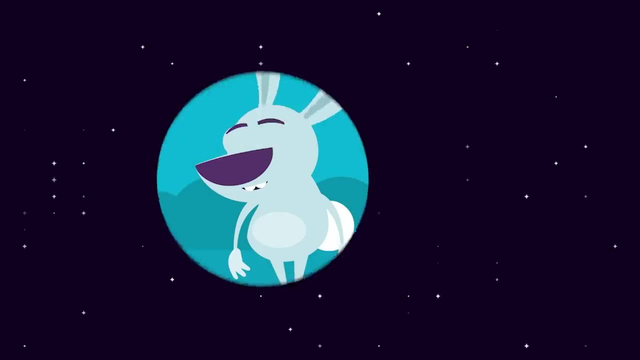 Joining your thumbs and fingers together. have a look through. Oh, look at that. Those colours, Those shapes, Oh, spinning around and around. Can you see it? Yes, it's a rabbit. It's Peter Cottontail, the Easter Bunny. 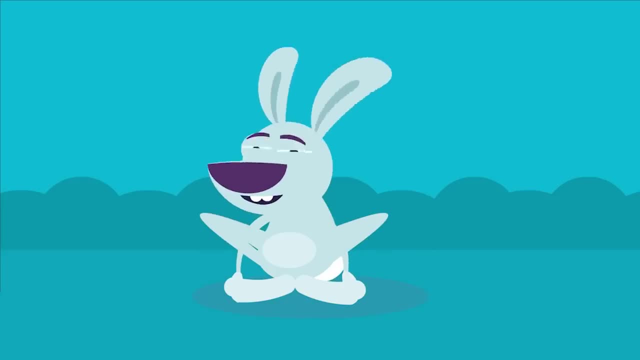 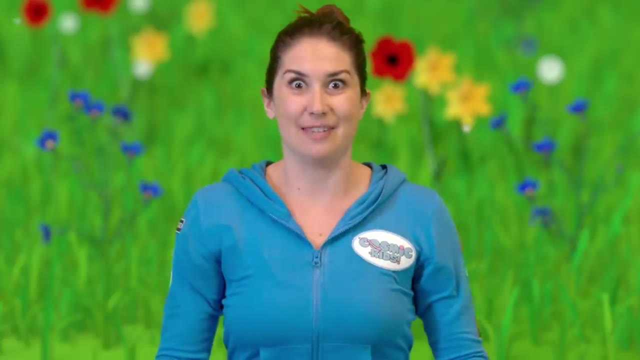 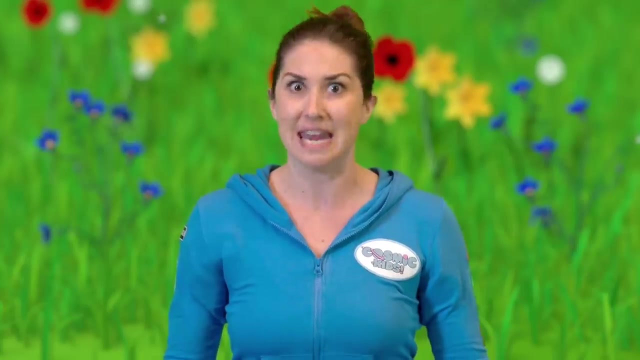 Hello Peter Cottontail. What's Peter doing? He's doing yoga. He's doing butterfly pose. This is very exciting. We're going to see Peter Cottontail, The Easter Bunny, and, with Easter coming very, very soon, he's going to be very busy at the moment, so maybe we can help him. 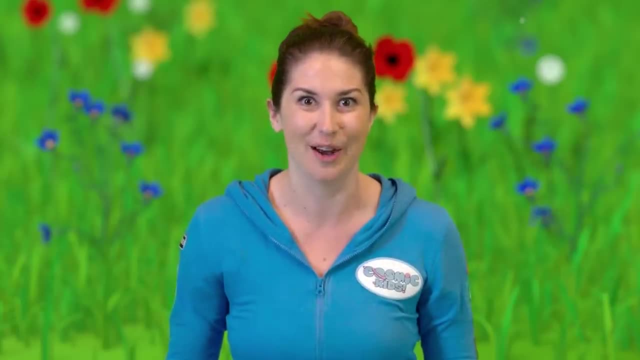 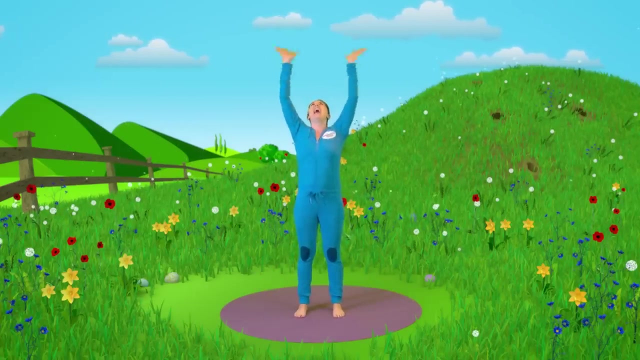 Let's get ready for our adventure by bringing out the sunshine. We stand up, we reach our arms to the sky and we say Hello sun, Ready, Hello sun. Then we fold all the way forwards and we say hello to the daffodils. 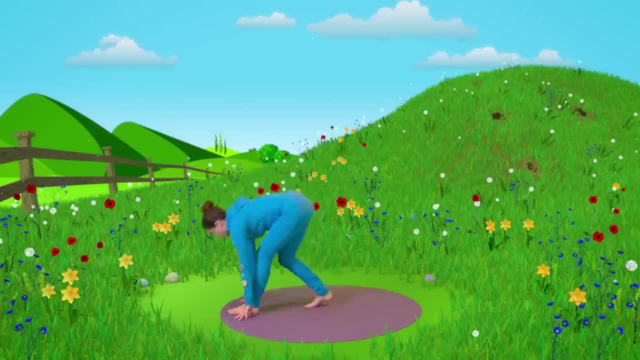 Hello daffodils. We step one leg over the other, We put one leg all the way back behind us and we drop down to our back knee. Then we lift ourselves up, Try not to wobble, We wrap our arms around and we go cheep, cheep, cheep, cheep, cheep, like little yellow chicks. 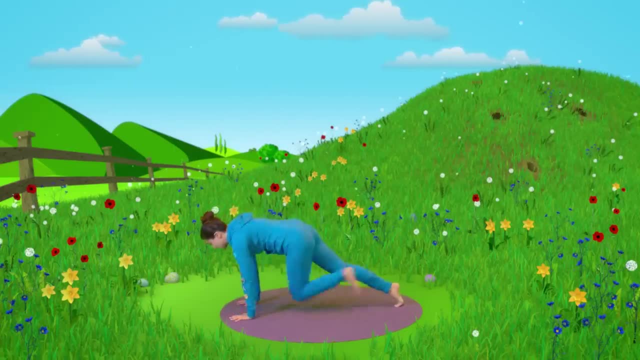 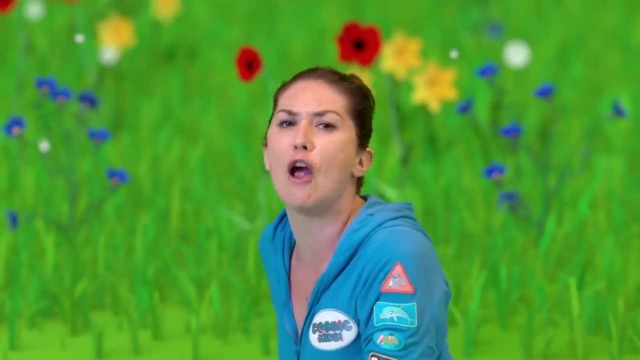 Very good. We bring our hands all the way down and we step our other leg back, coming down into our bellies. Then we wiggle, wiggle, wiggle, wiggle up like a very hungry caterpillar. Mmm, mmm, mmm, mmm. 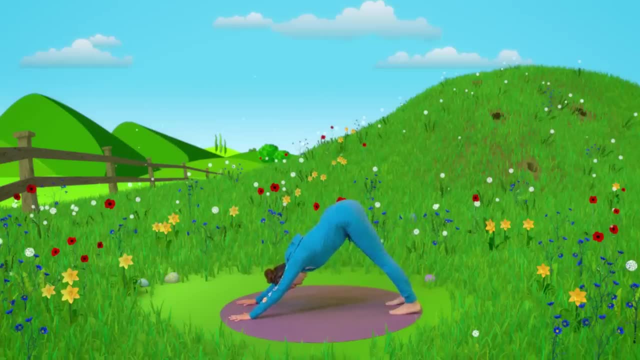 We tuck our toes, lift our hips up to the sky and we wiggle, waggle our little bunny tails. Then we step our other leg forward and we drop down to our back knee again. We come on up, trying not to wobble. 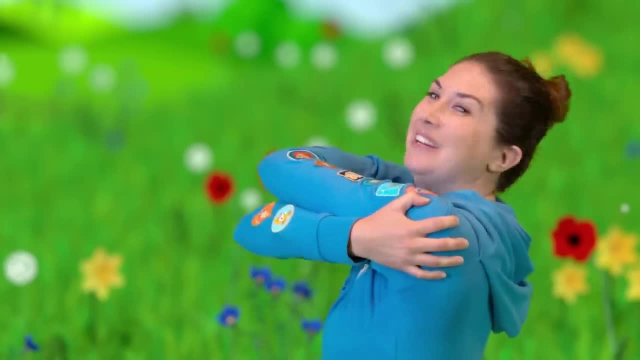 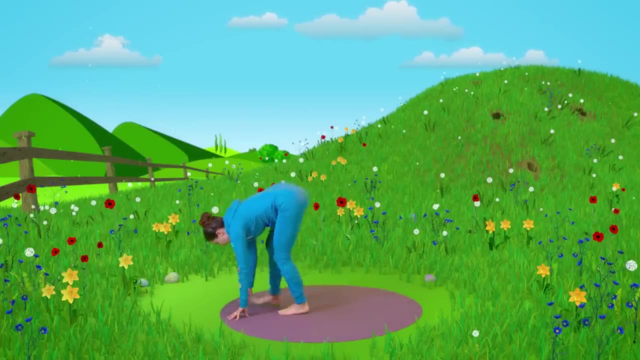 We wrap our arms and we go- cheep, cheep, cheep, cheep, cheep, like a little yellow chick. again, We take our hands down to our front foot and we step all the way forwards again to say hello to the daffodils. 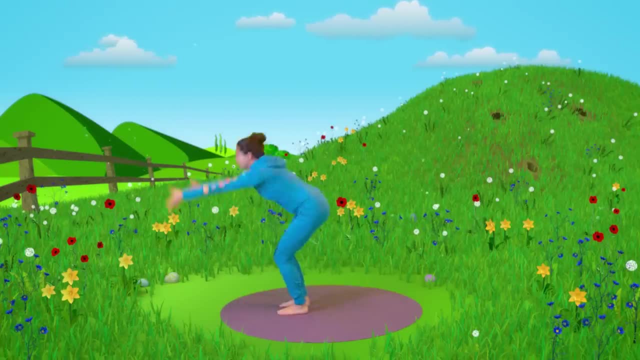 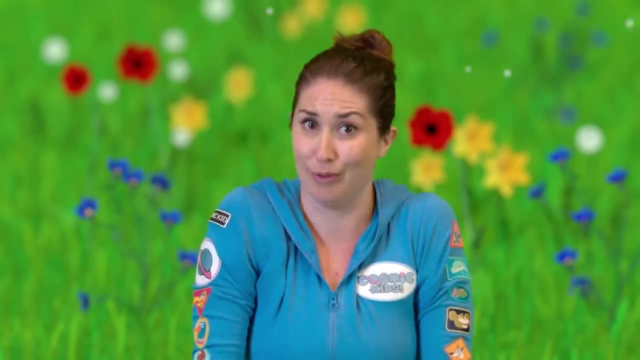 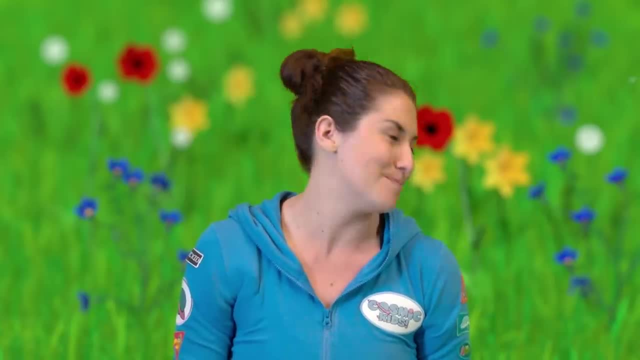 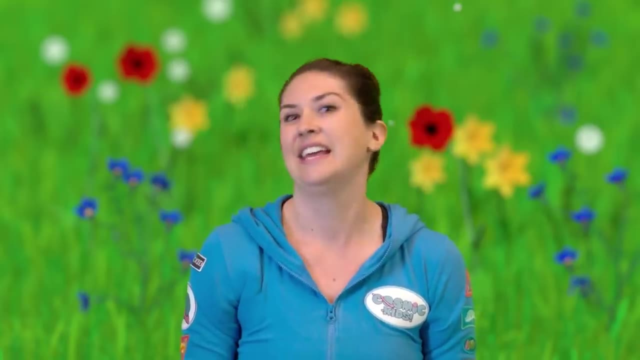 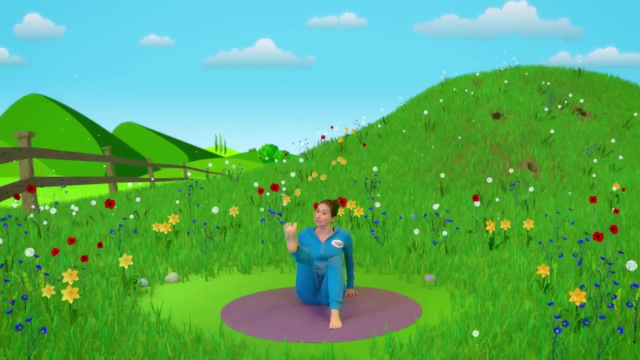 Very good, everyone. Now we roll our head around in a big circle one way and a big circle the other way. Getting our necks all nice and ready, We sit back on our bottoms, bring our hands behind us to help us balance. We lift up one foot. 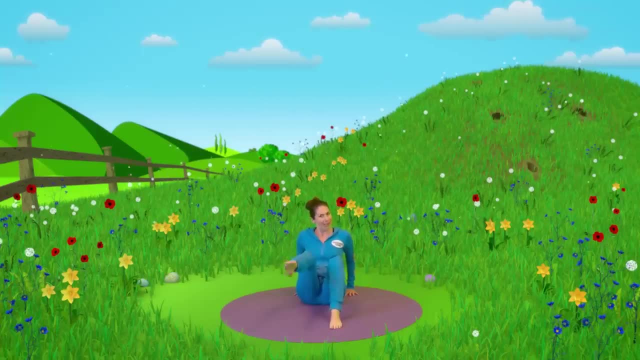 Then we go round and round in a circle with our ankle. Can we do the other one as well? We can. Now here's a challenge. Can we do one hand as well? You can? What about the other one? All four? 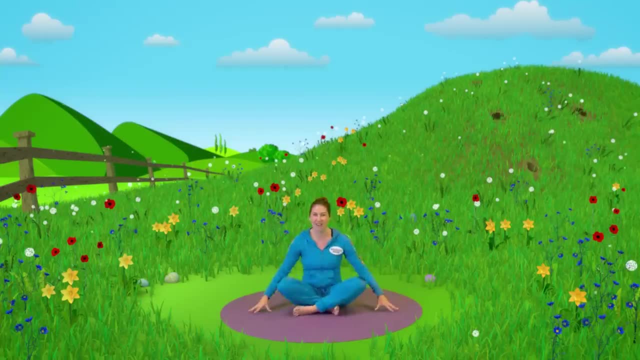 Well done everyone. That's brilliant. Now, crossing our legs Before we go: let's have some good breakfast, Let's have some porridge. We reach up high for the pot and we fold all the way forwards, Keeping our bottoms on the ground to put our pot in front of us. 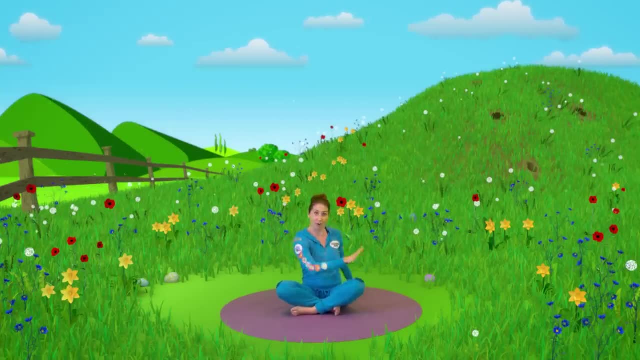 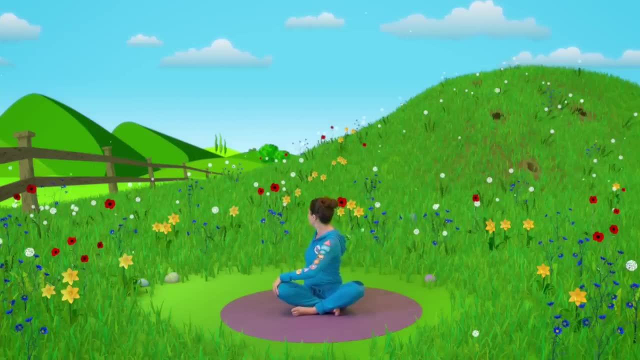 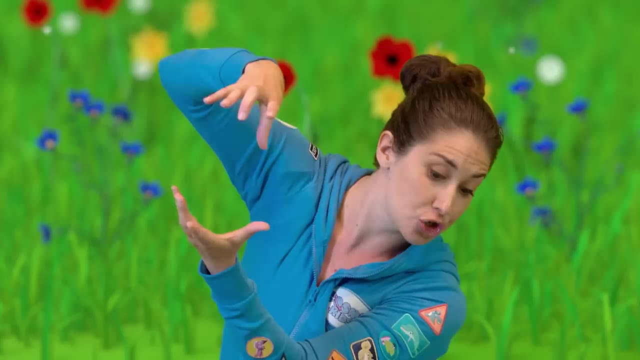 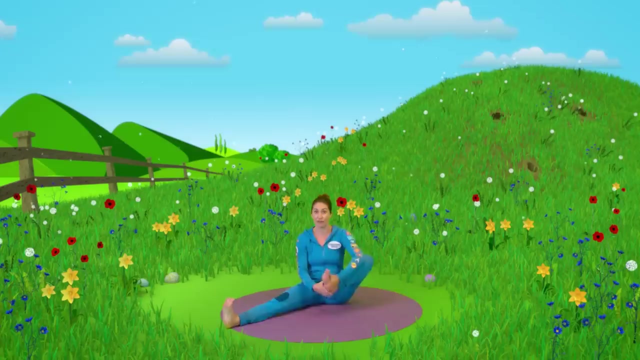 Then we take our other hand across to our opposite knee and we twist the other way round to get our water. Here it is, We bring it to the front and we pour it in Lovely. Now for the stirring. We take our legs out nice and wide and we take hold of one of our stirring spoons and we stir it up. 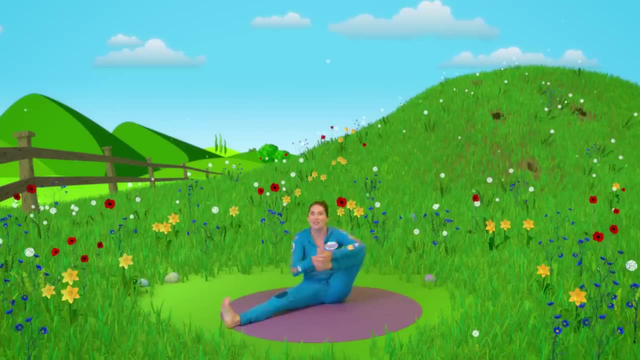 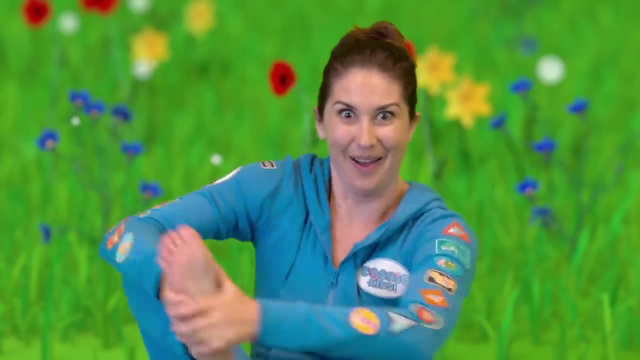 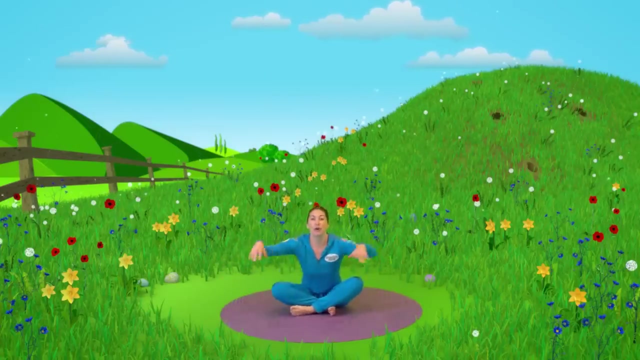 Very nice. Ooh, it's getting thicker. Let's try with the other one. now Take that spoon down and lift up the other one, Stirring it up. Very good, It's ready, Putting your foot all the way down, we cross our legs, fold forwards. 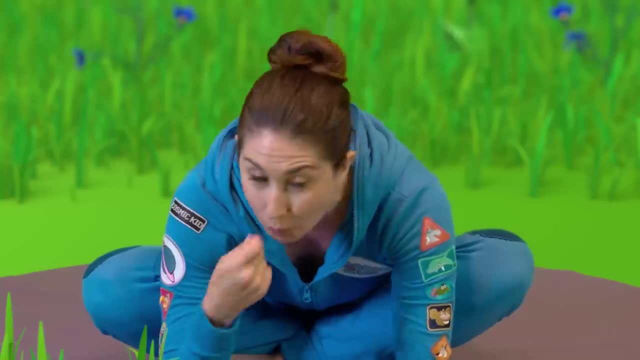 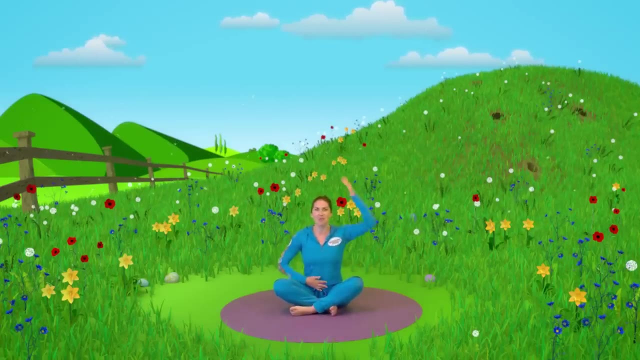 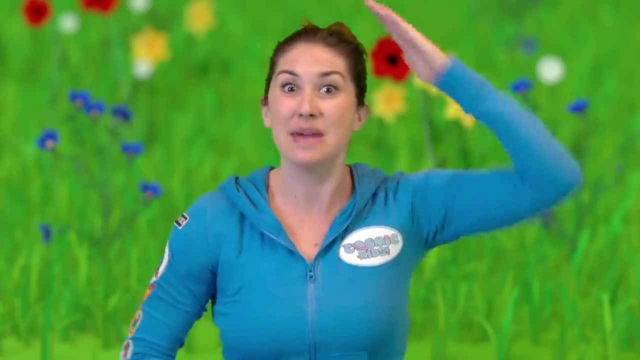 and we eat up all of our porridge. Mmm, it's delicious. We rub a hand on our tummies and we pat our heads at the same time. Very good, everybody. Now it's time to go and meet Peter Cottontail. 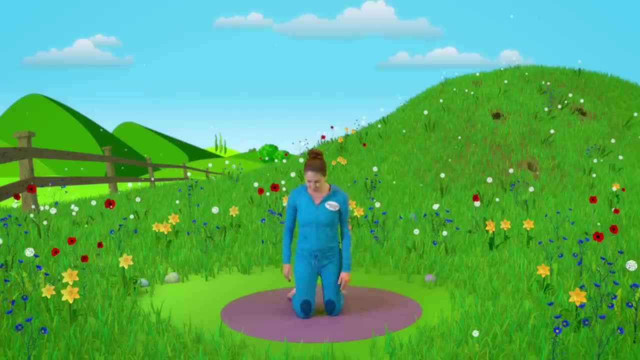 Let's go out the door, Coming to two knees- take your leg to the side and your arm up to the sky and we go vroom to open up the door. Now we need to go through the gate, Bringing your knees back together again. take your leg to the other side. 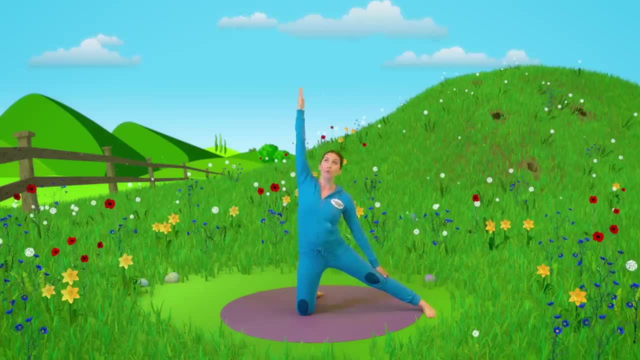 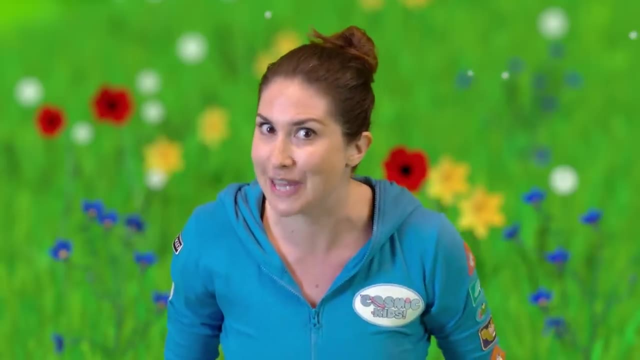 your arm up to the sky and open up the gate Vroom. Now we need to tiptoe down to the bottom of the garden so we don't scare Peter Cottontail. Shh shh, shh, shh shh. 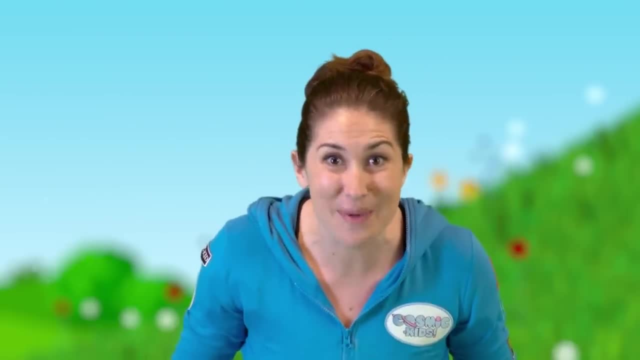 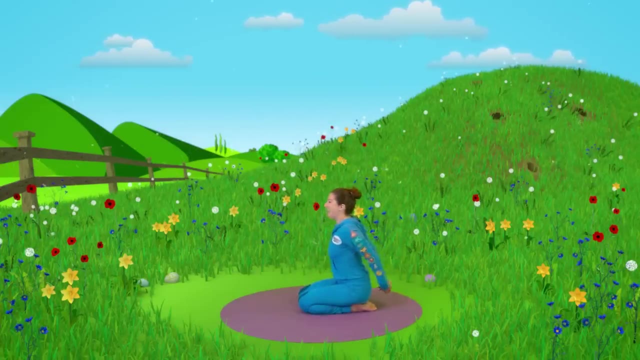 Look, here he is Waiting for us. It's Peter Cottontail. Come down to your knees and crisscross your fingers behind your back As you fold on forwards, lift your arms up above your head like two lovely bunny ears. 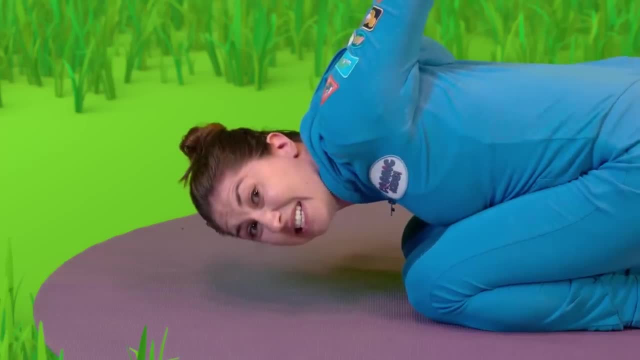 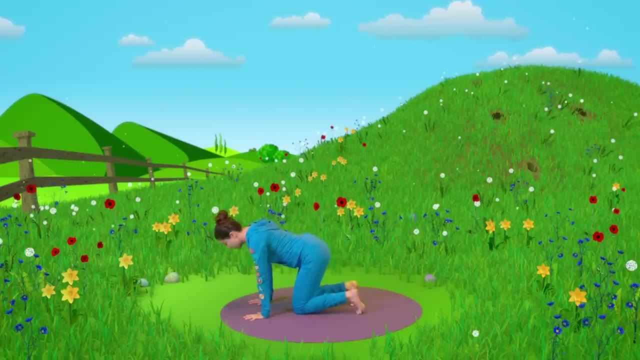 Peter Cottontail is so excited to see us. he does a couple of bunny hops Coming all the way up. put your hands down in front of you and tuck your toes, Lift up your bunny tail and go hoppity, hoppity, hop. 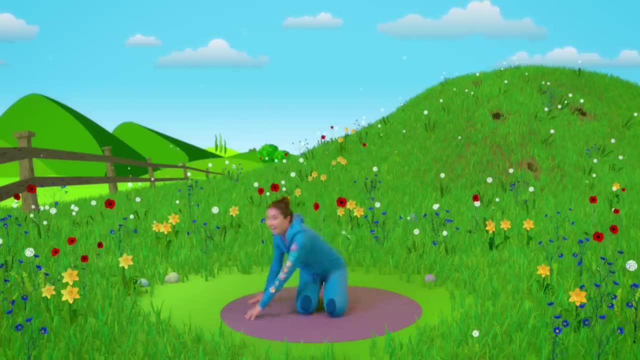 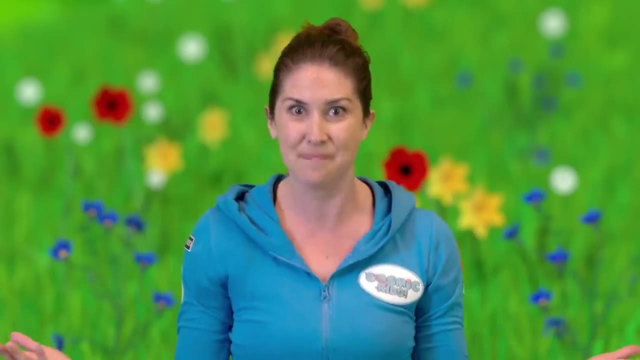 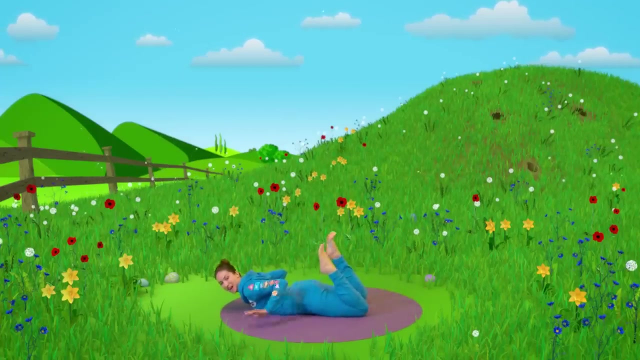 And again: hoppity, hoppity, hop. Wow, We're going to go and help Peter Cottontail, the Easter Bunny, collect lots and lots of Easter eggs for everyone at Easter. Let's grab a basket Coming down onto your tummies, we bring our feet towards our bottom and we reach around grabbing our ankles. 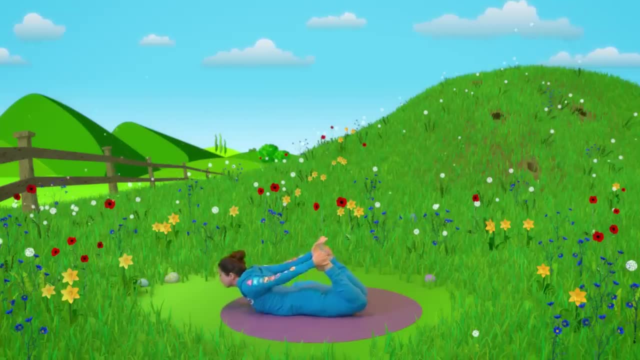 Then we lift ourselves up smelling the flowers- Ah lovely. Now time to get on our bicycles. We lower our legs and come back up to sit and take ourselves all the way down onto our backs. We crisscross our fingers and put them behind our heads and lift up our legs. 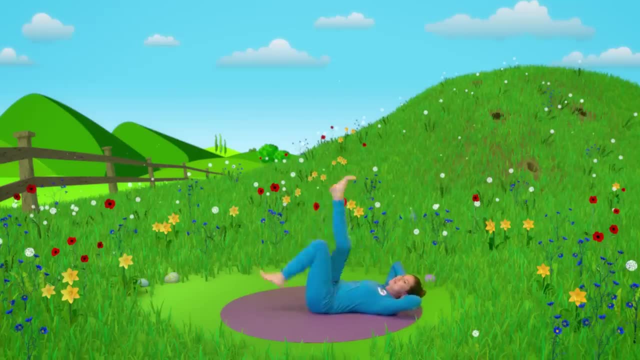 And we start to use our feet to do the pedals. We're going to have to collect lots and lots of eggs so that Peter Cottontail, the Easter Bunny, has plenty for everyone. Look, we've arrived in the woods, Coming up to stand. 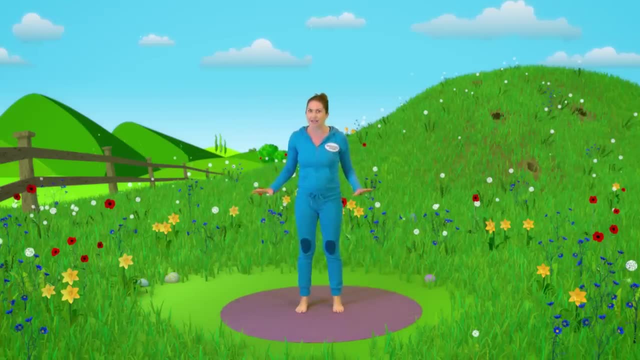 We need to see where to go first to go and collect some eggs. So let's climb a tree Here. we go Up, we go up, we go up, we up, we up, we go. Ooh, is this high enough? Let's see. 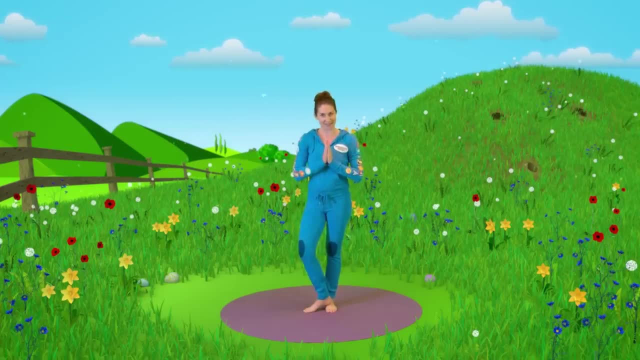 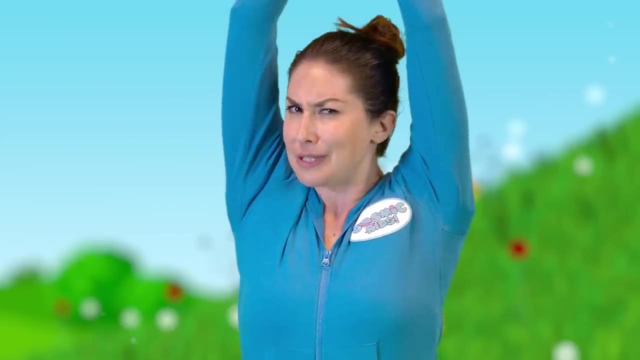 Bringing one foot on top of the other and your hands together at your heart. Grow your tree up nice and tall. Ooh, now, hang on a minute. Are you a strong tree today? Do you think I can blow you down? Mmm, I think I can. 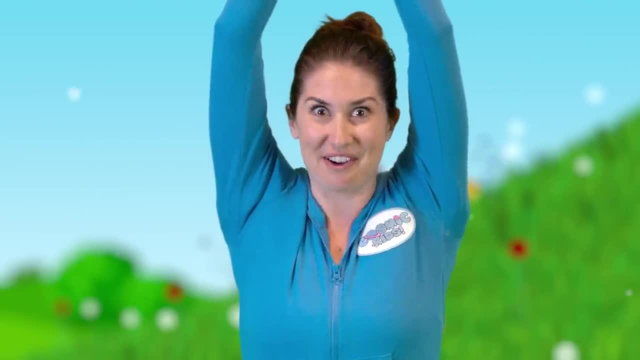 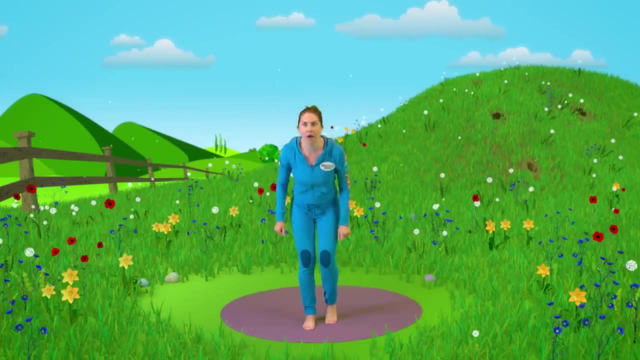 Let me try. You stay tall and strong. I'll have a go. Here I come. I don't believe it. You're still standing up. You are super duper strong. Let's climb a bit higher and see how we do up there. 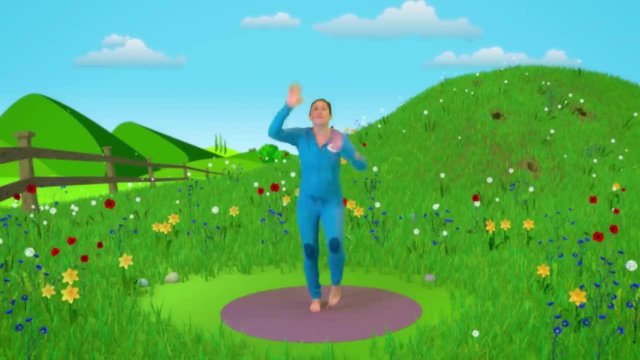 Ready Up, we go, up, we go up, we up, we up, we go. Let's try our tree on the other side now, Bringing your other foot on top, Your hands together, And grow up nice and tall. Ooh, try not to wobble. 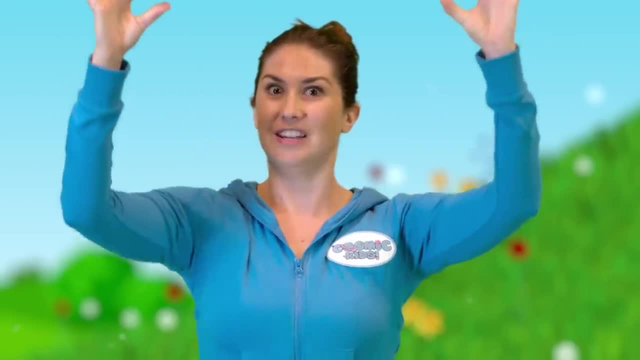 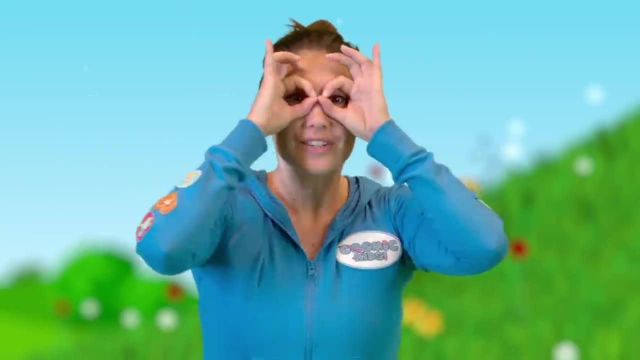 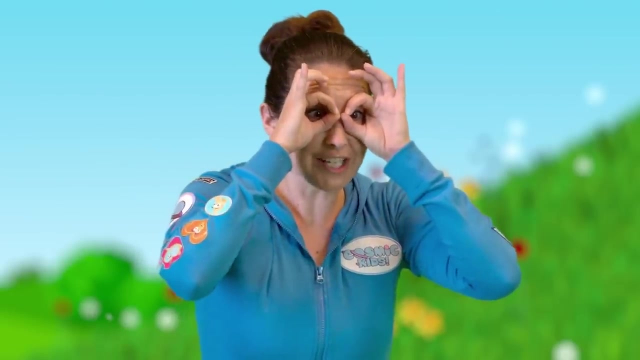 Now I wonder if you can make your fingers into binoculars, joining your thumbs and fingers together. Have a look through. Ooh, look, Trying not to wobble, We're very high up here. Look down there, It's Tommy the bedtime turtle. 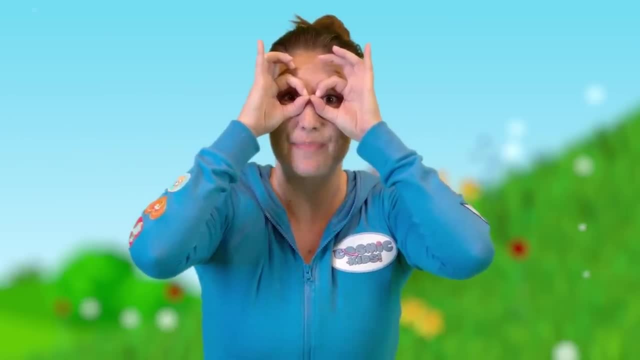 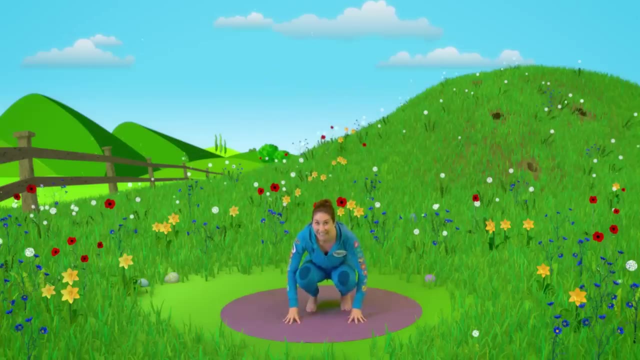 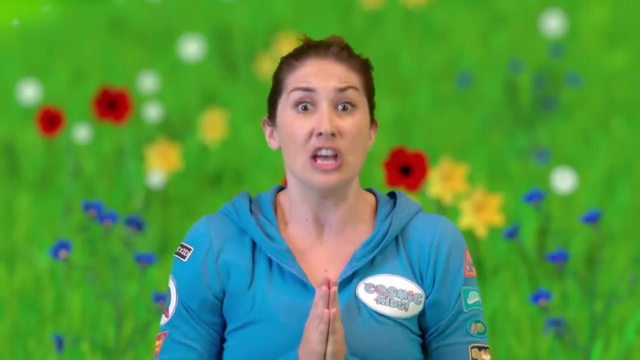 Maybe he'll have some Easter eggs for Peter Cottontail, the Easter Bunny. Let's jump down and ask politely: Ready, One, two, three Boing. Peter Cottontail asks very nicely. Oh, hello, Tommy. Please may we have some Easter eggs for Easter? 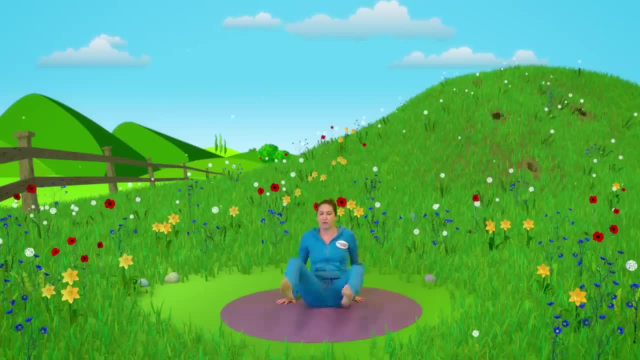 Coming into our turtle position. we sit on our bottoms and bring our feet in front of us, bending our knees. We bring our hands down in between our legs and shuffle them underneath our legs, making a pair of turtle flippers. Tommy lifts his head out of his shell. 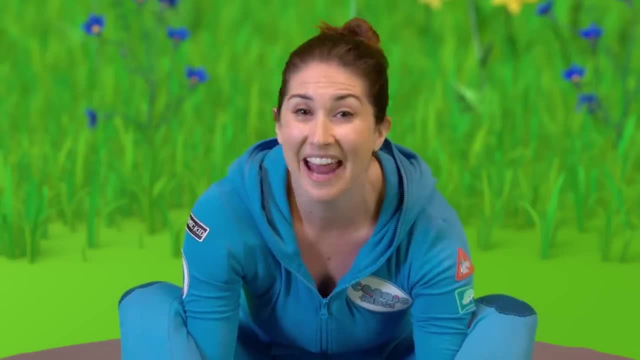 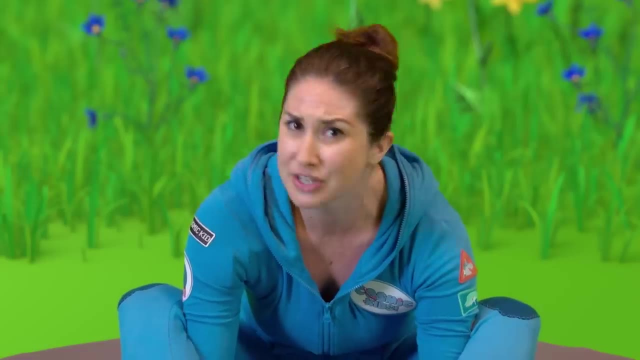 and gives us a great big smile: Hee, hey, there. It's so good to see you And seeing as you asked me so nicely and you said: please, of course you can have some eggs for Easter, But I'm afraid I only have one. 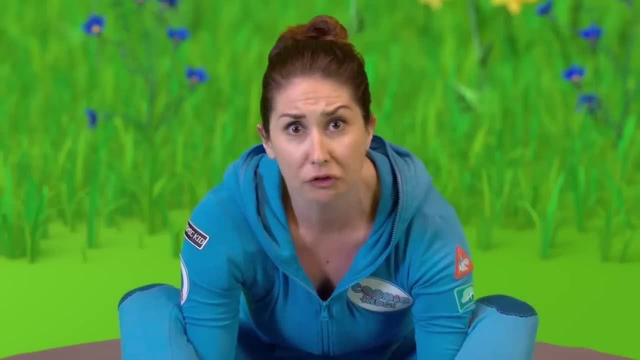 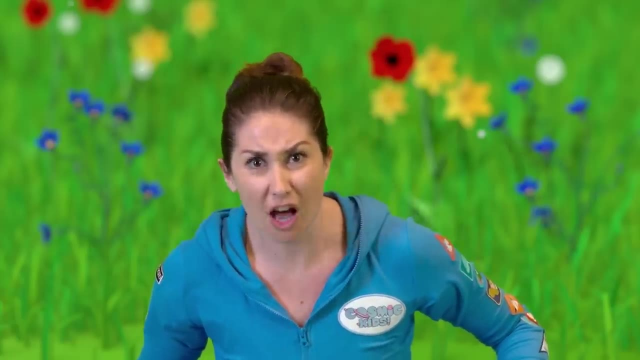 I seem to have lost all of the others. I don't know where they've gone. We come up to sit and cross our legs. Hmm, that is funny. Where on earth could the other Easter eggs be? We say namaste to thank Tommy. 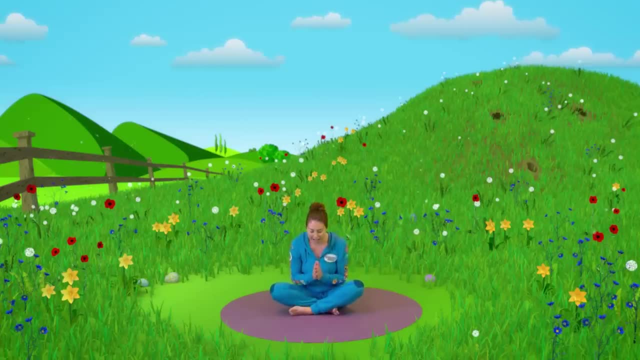 One, two, three, Namaste. We come to a lake where there's a little boat waiting for us Coming to sit round. lift up one leg, lift up two. lift up one hand, lift up no hands. Yay, give me a wave. 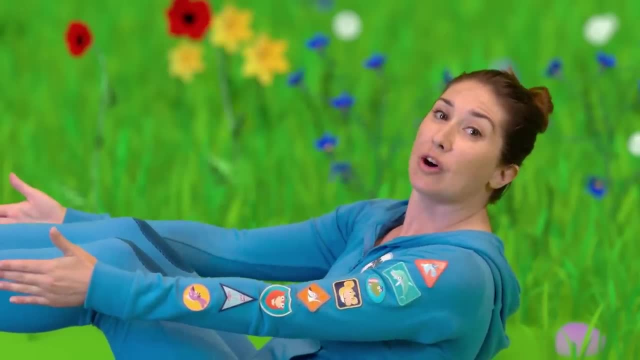 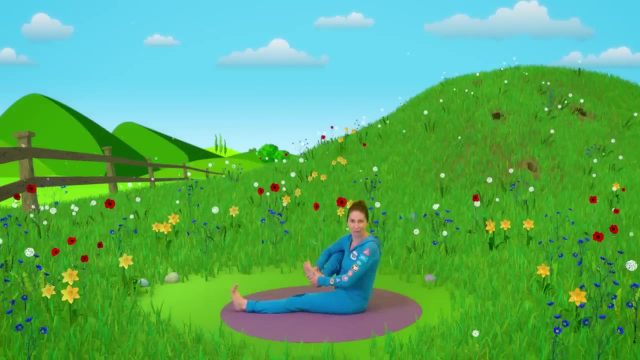 We're in our boat pose And with Peter Cottontail, we row. Take your legs out long, Take hold of an oar And let's sing our row row, row your boat song. Ready Row, row, row your boat. 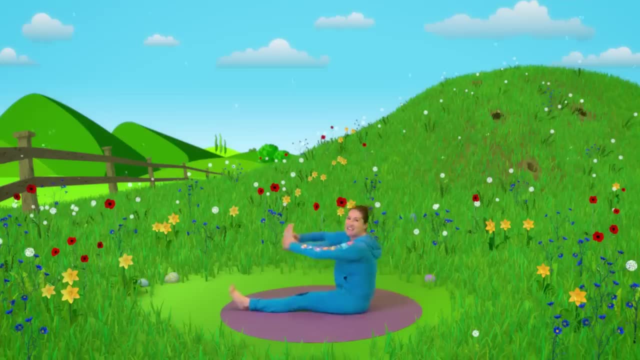 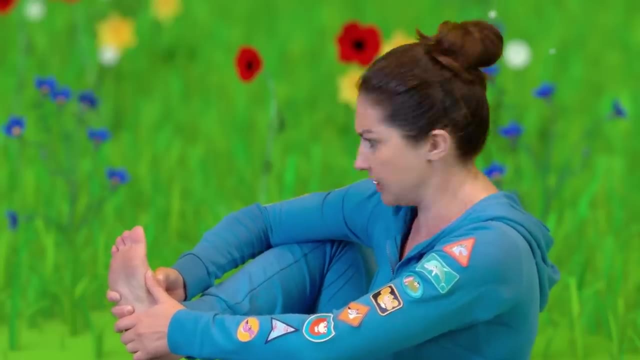 Gently down the stream, Merrily, merrily, merrily, merrily. Life is but a dream. Ring, ring, Ring, ring. That's his telephone. Shall we answer it, Okay, yeah, Hello, Oh, it's Belinda the hen. 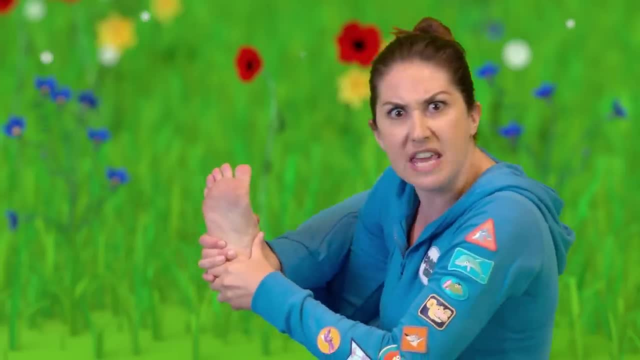 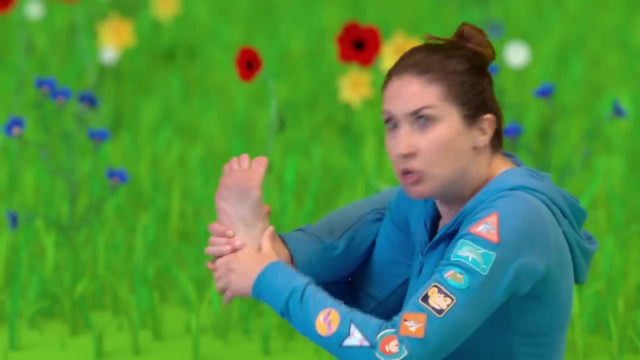 Hi, Belinda, What? All of the Easter eggs are gone, But, but, but, but, where? Oh, okay, Belinda, Speak to you soon. Bye, We put the phone down. Where could they have gone? We need to keep rowing, so we pick up the other oar. 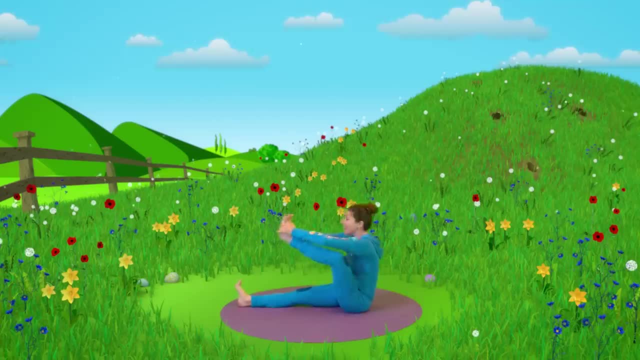 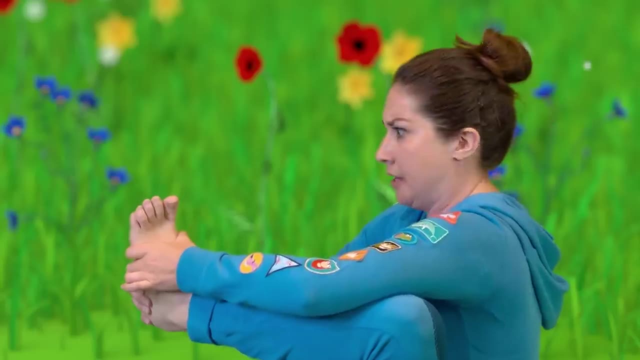 Row, row, row your boat Gently down the stream, Merrily, merrily, merrily, merrily. Life is but a dream. Ring, ring, Ring ring. That's the phone again, Let's answer it, Hello. 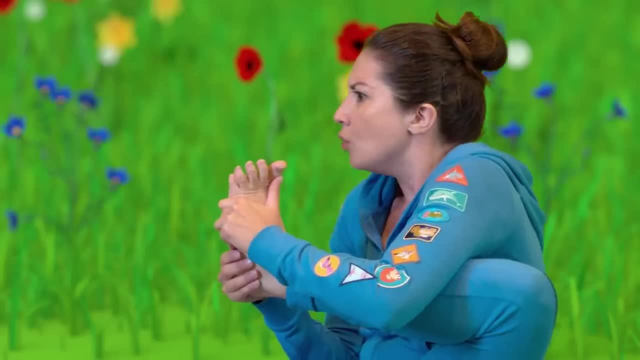 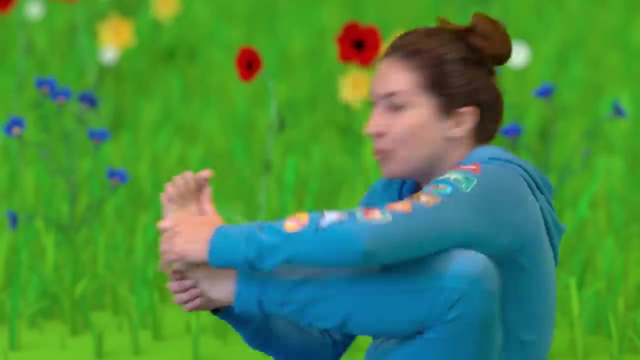 Oh, it's Belinda again. Hi, Belinda. Oh, we've got to speak to Colonel Crockles the crocodile. Okay, Right, Thank you, Belinda. Bye, We put the phone down and we come face to face with a crocodile. 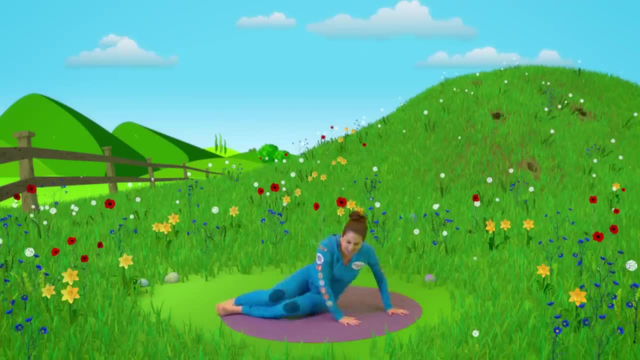 This must be Colonel Crockles, the crocodile, Lying on your side. take your arms up long above your head and open and close your jaws like you're a snappy crocodile. Let's see if we can swish our tail as well. 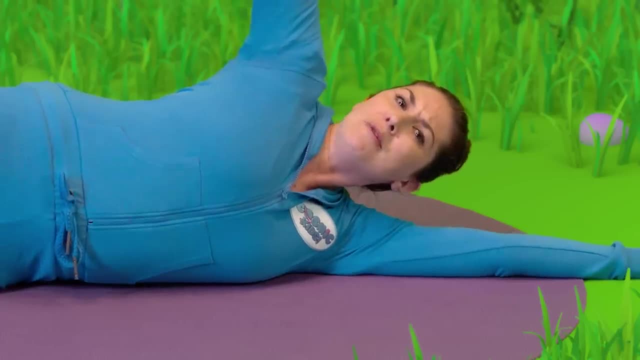 Oh, very good, everyone. I tell you everyone, it's those tricksy tickly monkeys. They've gone and stolen all the eggs and they're hiding them in the back of their cave. They simply don't want to share them with anyone Coming up to sit. 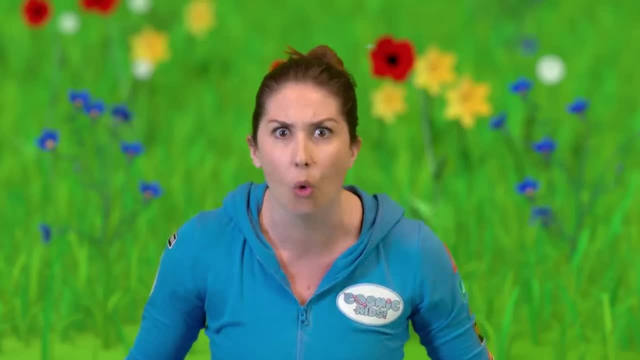 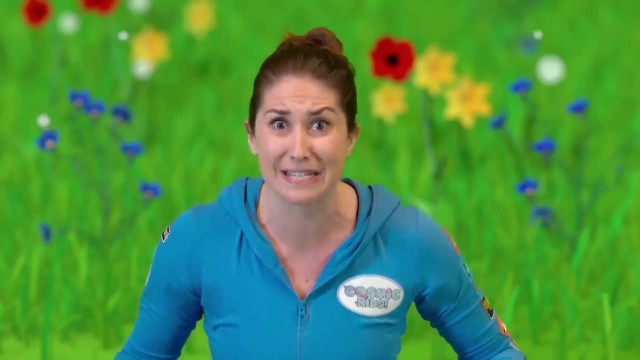 We cross our legs. Oh no, This is awful. If those tickly monkeys have stolen all the eggs, then there won't be any left for everyone at Easter. What are we going to do? We know what to do. We're going to take some deep breaths. 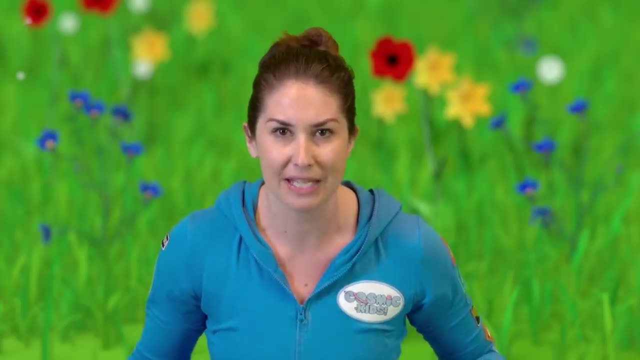 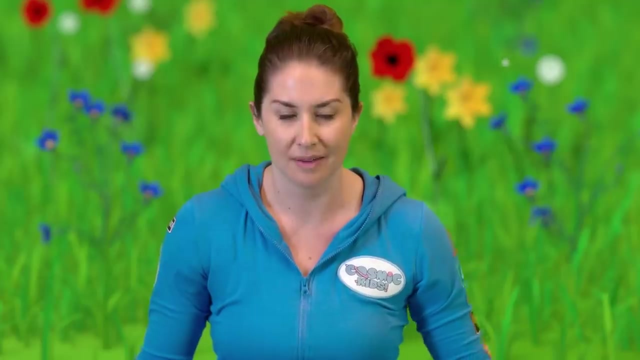 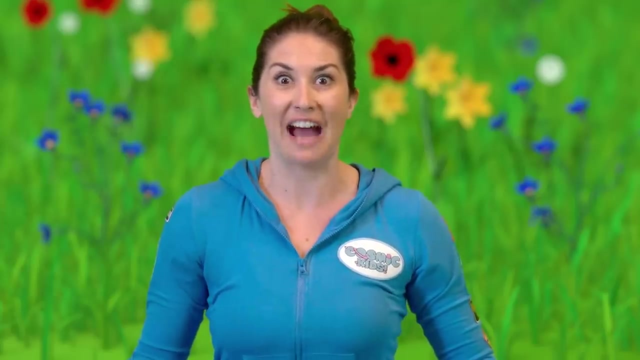 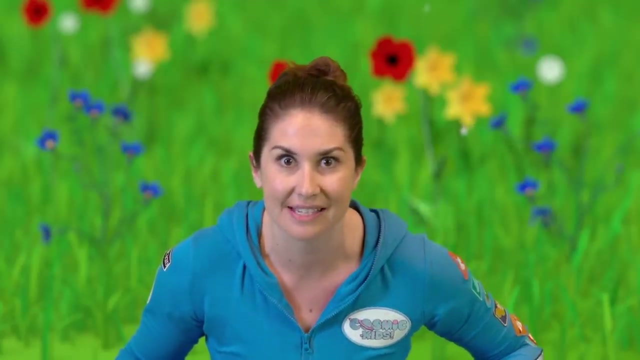 We're going to calm our minds down and we're going to have an idea Ready. We've got it. We've hatched a plan to save the eggs. Let's all pretend to be eggs, Then, when the tickly monkeys come, they'll think that we're eggs and they'll come and pick us up. 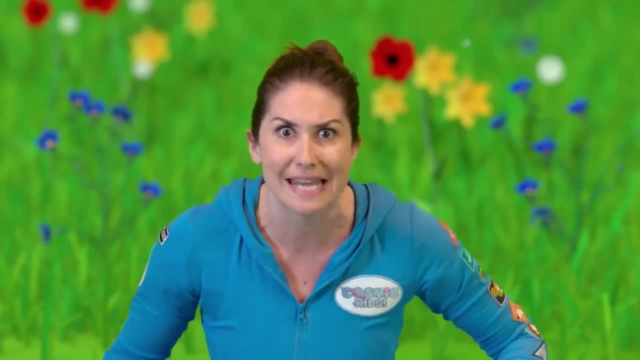 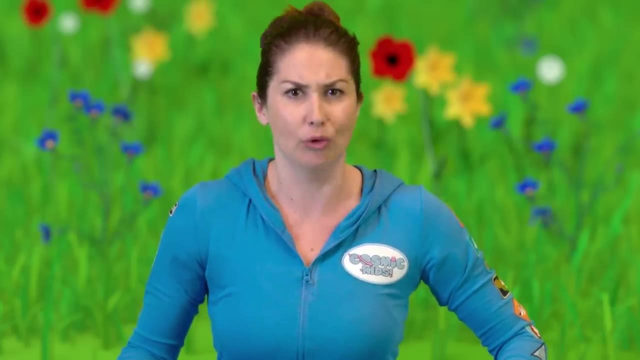 and add us to their collection. Then we can wait until they've gone to sleep and we can collect all the eggs and take them out. We can rescue them. This is a brilliant idea. Colonel Crockles agrees? Lying down on your other side now? 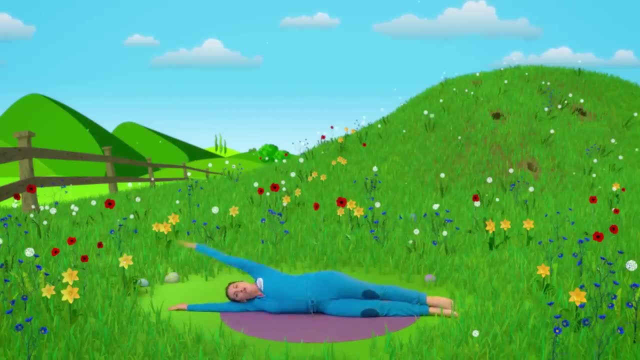 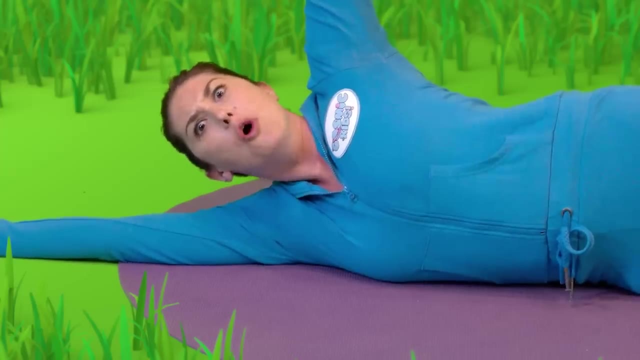 stretch your arm up above your head and open your snappy jaws And let's do some tail swishing on this side, And let's do some tail swishing on the other side too. Perfecto mundo, Cosmic kiddos. Thanks, Colonel Crockles. 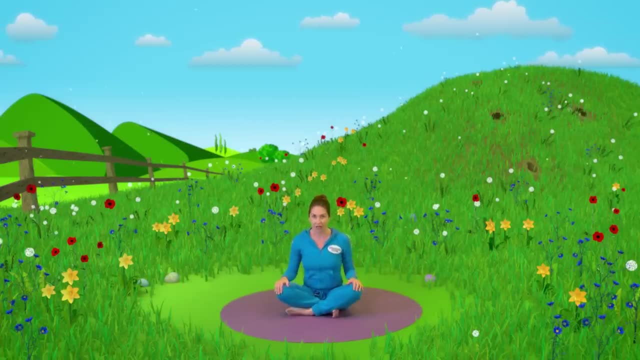 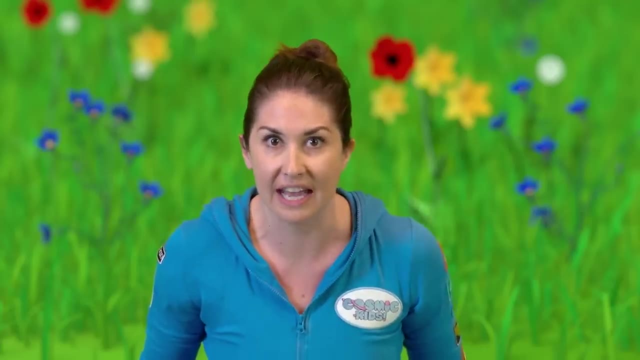 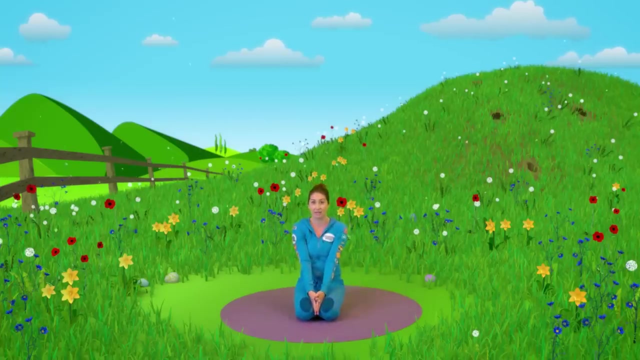 We sit on up and we get ready to go to the cave where the tickly monkeys are living with all of the eggs. On the way, we hear an owl twit to wooing to warn us Coming to your knees. draw your hands down in between. 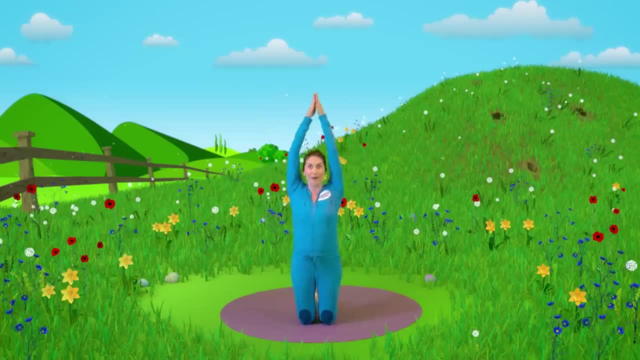 We lift up as we go twit, and lower as we go twoo and again twit, twoo. Be careful, there are tickly monkeys in there who like to tickle you. We say Namaste to the owl to thank her. One, two, three. 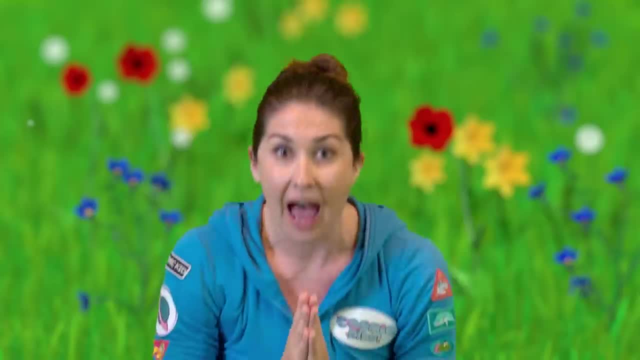 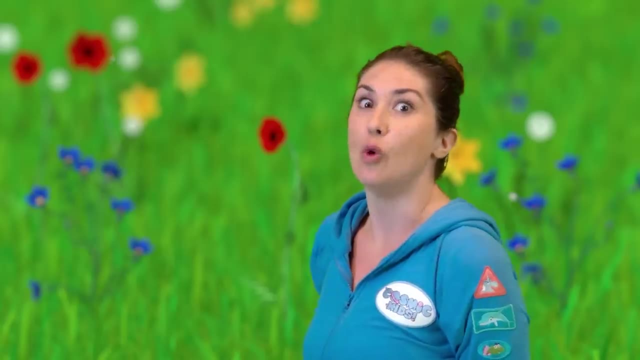 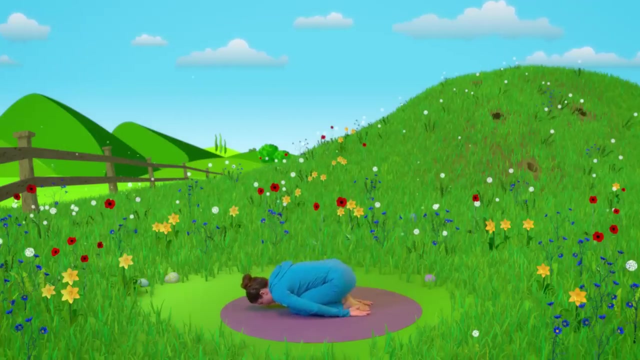 Namaste, And we get ready to look like little little eggs Coming to your knees. we're going to be like little eggs that have fallen over in the grass, Folding yourself all the way forwards. We wait for the tickly monkeys to come and find us. 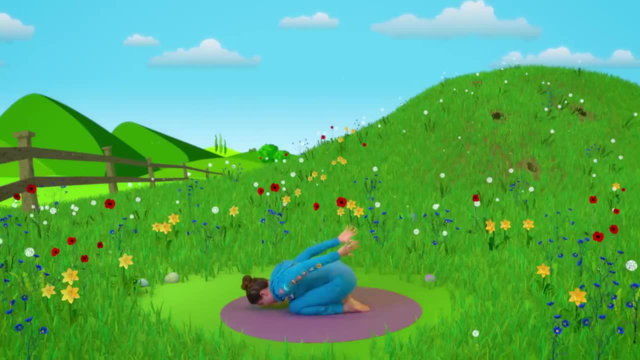 Here they are, Bringing your hands up, wiggle your fingers and pitter patter on your backs. The tickly monkeys are taking us and they're putting us in their cave with the other eggs, Keeping very, very still. After a while we hear a noise. 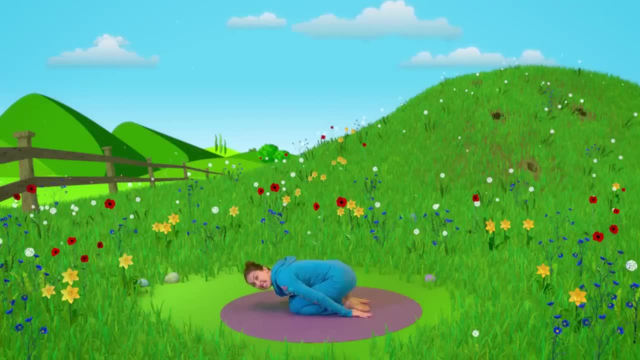 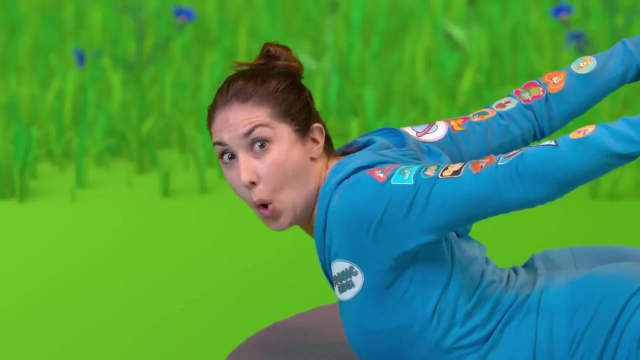 It's the tickly monkeys. They've gone to sleep. Quick, get your basket coming onto your belly, Bring your feet to your bottom, Reach around and lift yourself up into your basket. pose. Now we collect all of the eggs and we get them out of the cave. 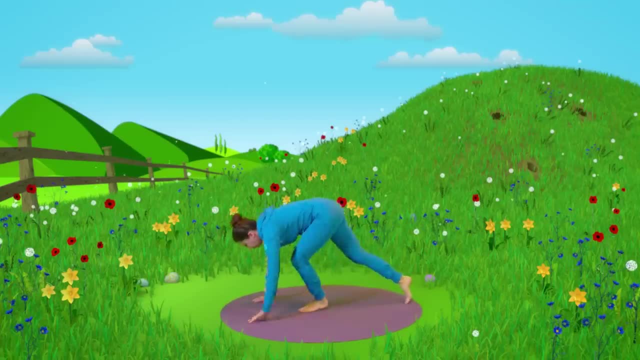 Come on, everyone standing up, Up we come. We tiptoe, tiptoe, Very quietly out of the cave. What's that? It's alright, It's just a little spod the spider, Bending your knees and bringing your fingers in between your feet. 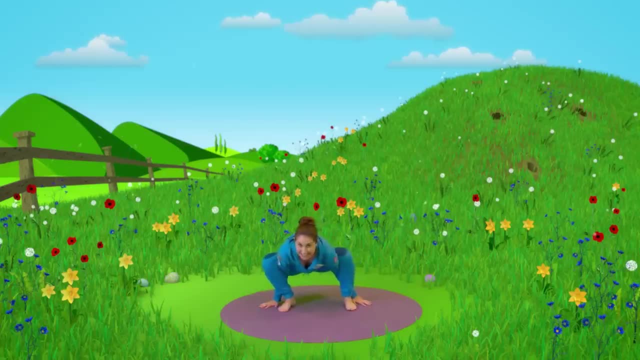 we go tikka, tikka, tikka, tikka, tikka to the outside. Oh, sorry about that. We carry on tiptoeing out of the cave, Coming up to stand, Tiptoe Shh, shh, shh. 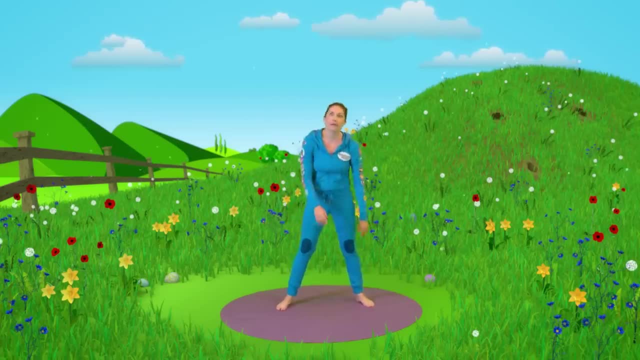 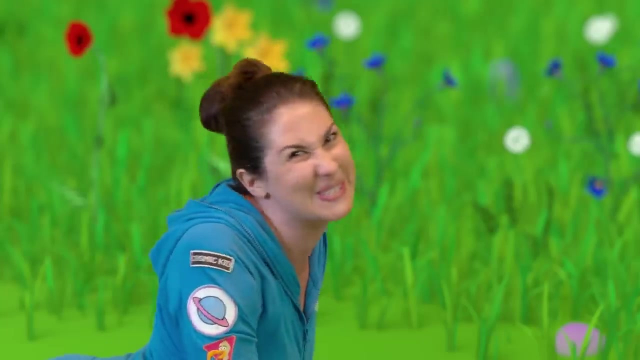 What's that? Oh, it's okay, It's just a little sessel, The slithery snake Coming down onto your bellies. everyone Hands under your shoulders and sorry about that, Didn't mean to disturb you. We carry on tiptoeing out of the cave. 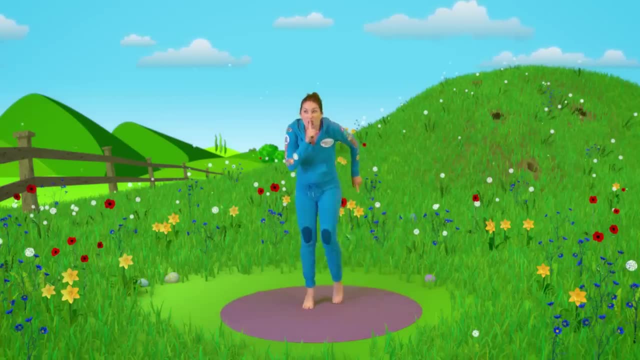 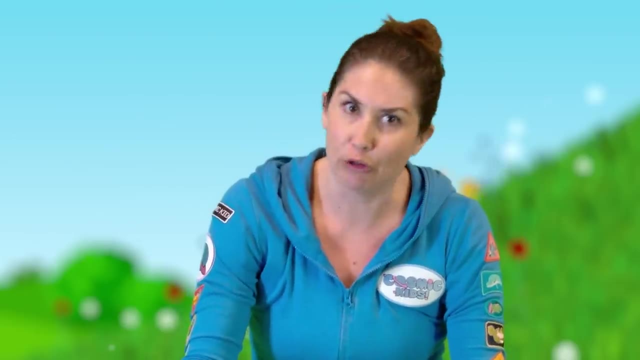 Up, we come. Shh, shh, shh. What's that? Oh, it's okay. It's just a little meldrum, the mouse Coming down onto your knees and tuck yourself up into a tiny little mouse ball. 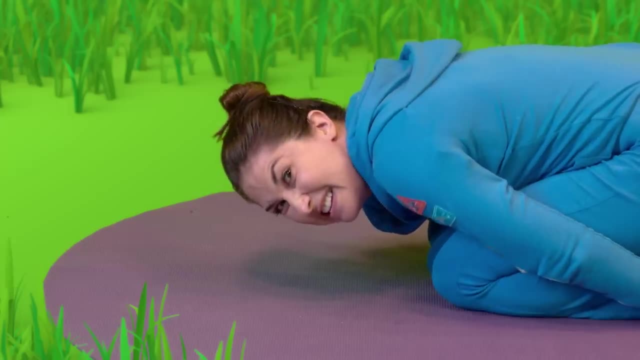 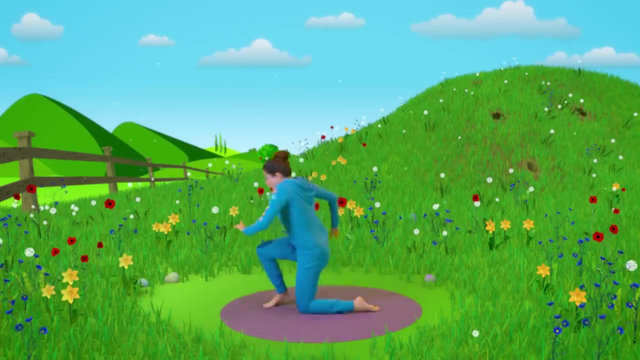 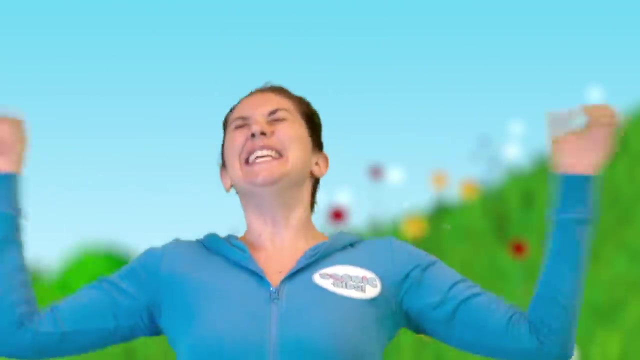 Squeak, squeak, squeak, squeak, squeak. We carry on tiptoeing. We're so nearly there. Up we come, Shh, shh, shh, And we've done it, Yay. 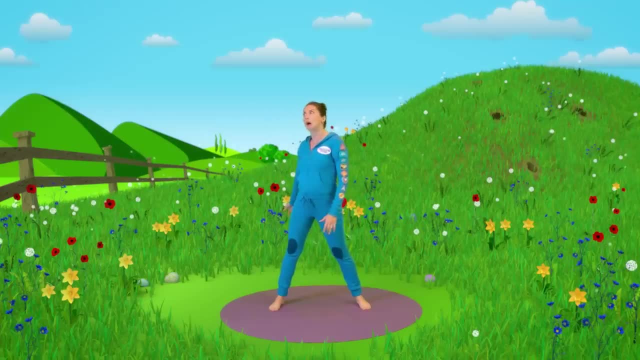 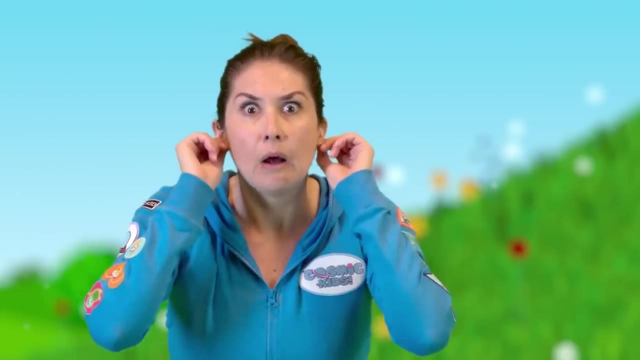 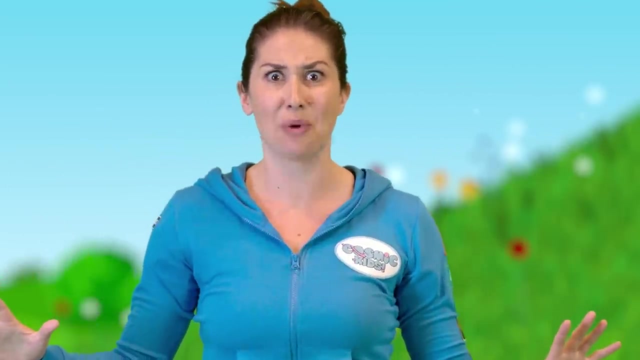 We wipe our brows- Phew, But what's that We can hear Rubbing our ears? It's the tickly monkeys. They've woken up and they're jumping into action, Crouching down on your toes, everybody, We're going to do a big monkey jump into the air. 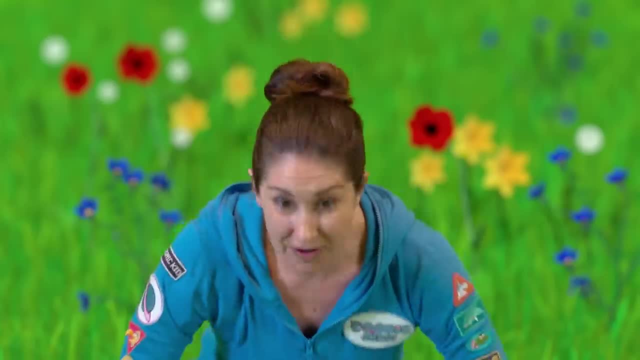 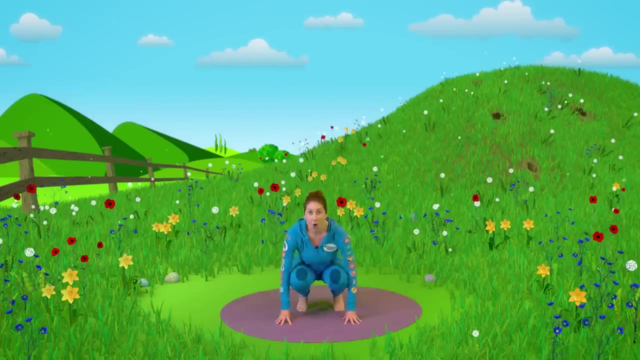 After three: One, Two, Three And again One, Two, Three. Quick Hide, Jump down the rabbit hole, Turning yourself around Hands down, Tuck your toes, Lift your bottoms up to the sky. This is a special rabbit hole. 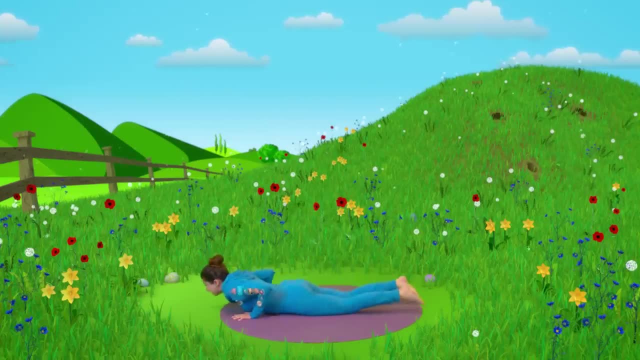 A rabbit warren In. we go on our bellies Slithering like snakes. Ooh, We're wiggling inside And we hide like little mice, Tucking all the way back with our arms and our head down. Shh. 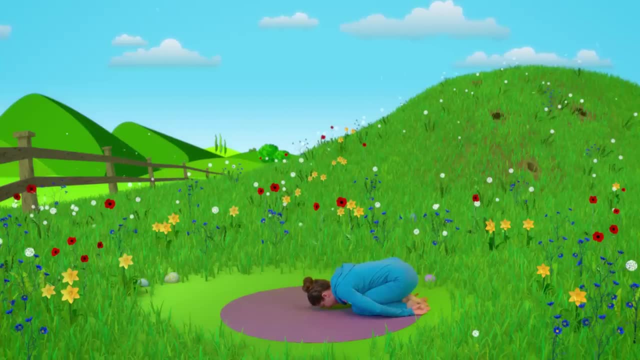 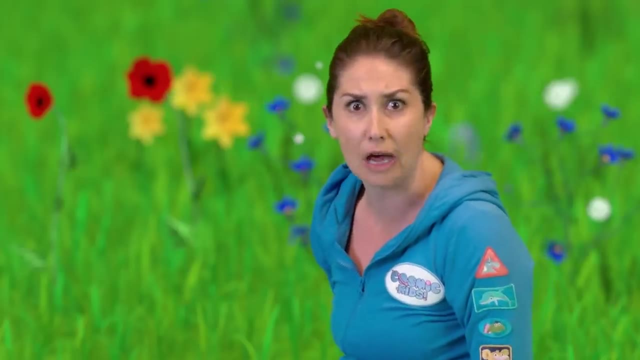 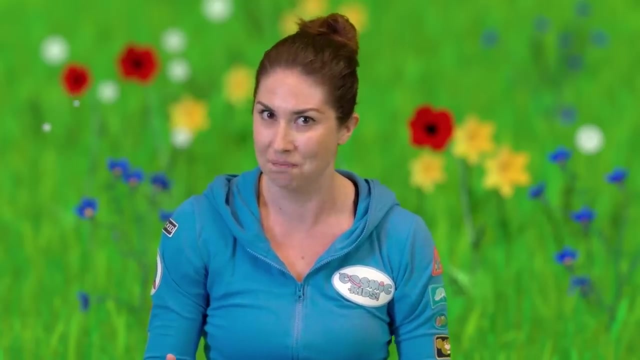 The tickly monkeys go running, Running past, And we sit up And we say, Phew, That is a relief. Peter Cottontail, Who is the Easter bunny, remember, Is actually quite magical And he crosses his legs. 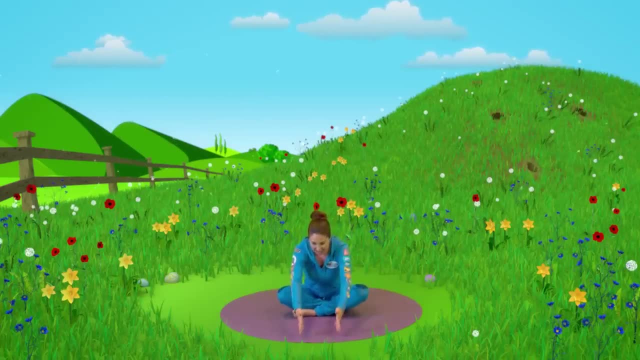 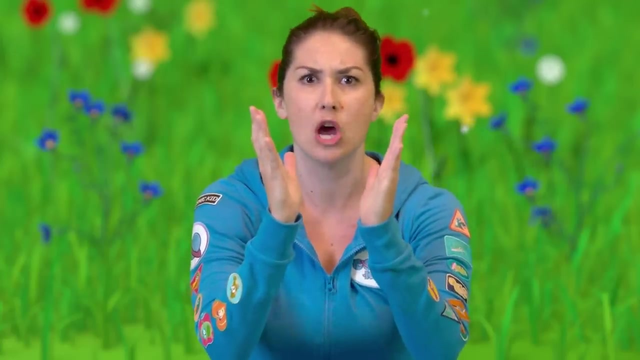 He takes one of the Easter eggs And he turns it upside down And when it's this shape, It looks a bit like a balloon And he says some magic words: With Easter coming so very soon, Let's turn this egg into a hot egg balloon. 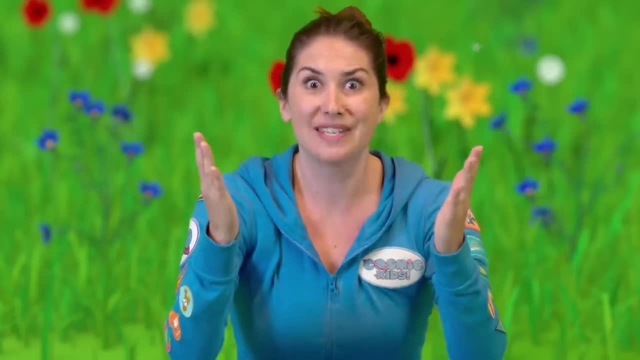 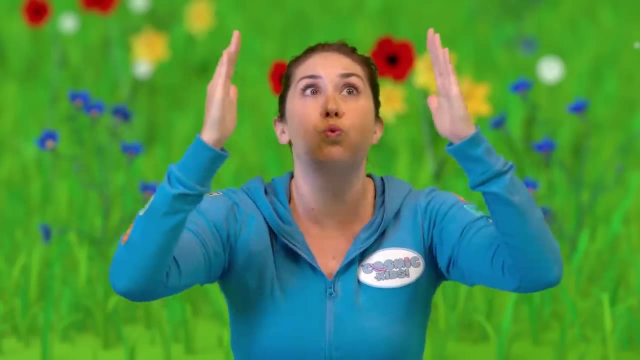 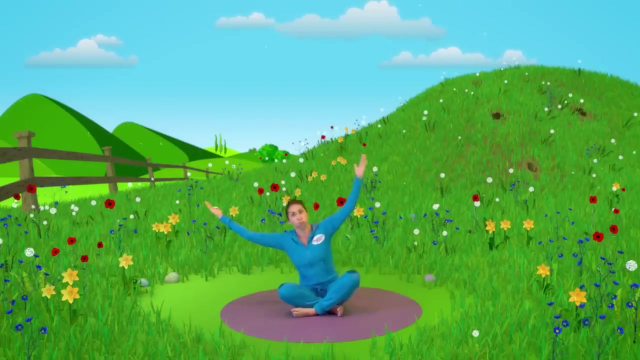 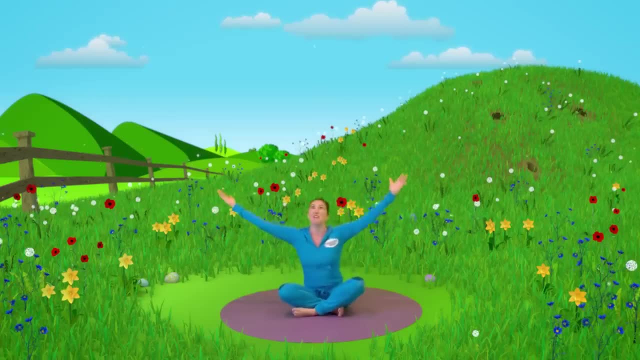 Wowzers, Look how big our balloons are. We're floating up into the sky above the woods, Away from the tickly monkeys, And we're heading back towards our garden with Peter Cottontail And all of the Easter eggs. We say our rhyme: 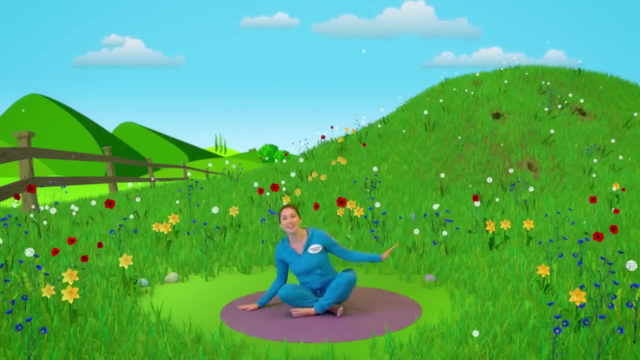 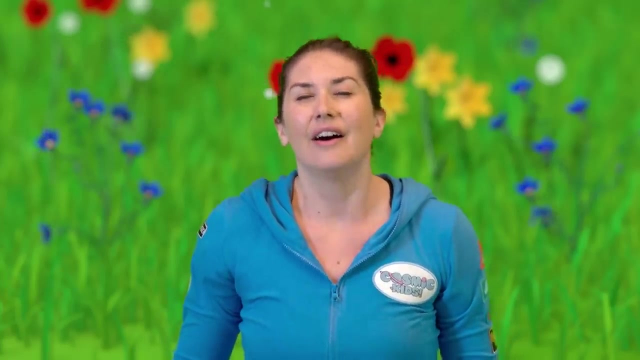 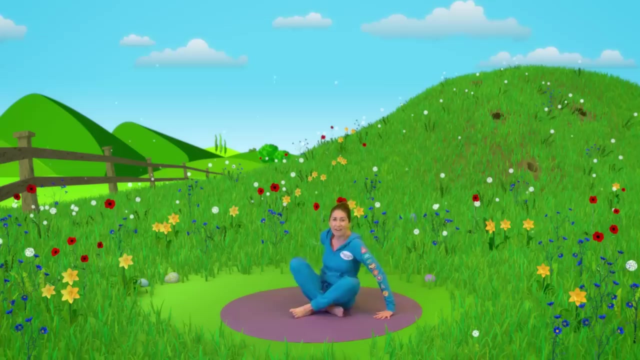 Tick Tock Like a clock, Until I find My sen Tra Ta. We found our centre, And we found ourselves back at home. Oh, We feel so exhausted, And so does Peter Cottontail, So we very quietly and very gently all get into our beds. 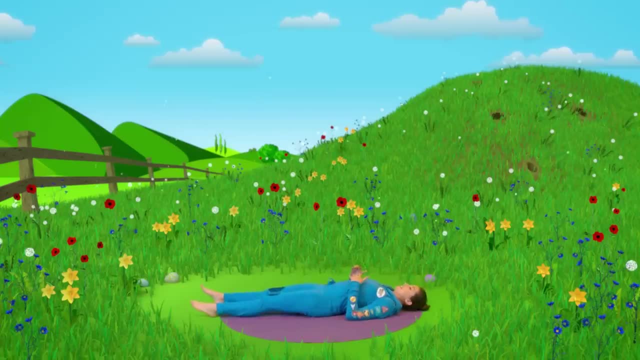 With Peter Cottontail snuggling up, He lies on our bellies And we gently stroke his lovely fur. He feels so good And we all get up, And we all get up. He feels so soft. we watch as his little eyes begin to close. 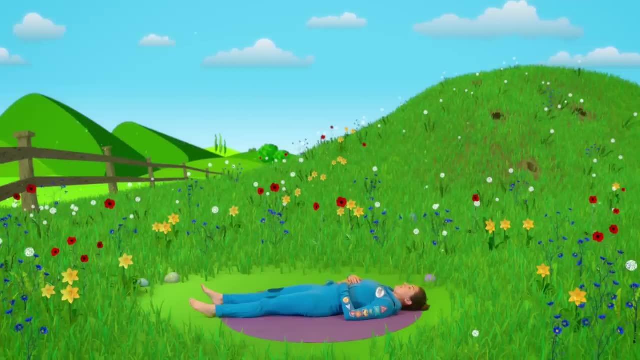 and his nose and his whiskers start to twitch as he is beginning to dream. Oh, it's so good what we've done today. We feel really proud of ourselves Helping Peter Cottontail rescue all of those Easter eggs from the tickly monkeys who just didn't want to share them. 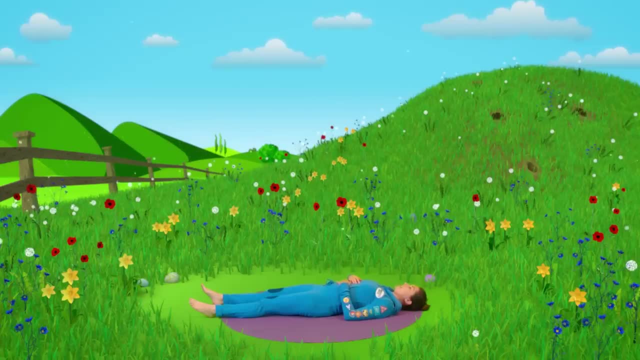 They were being very greedy, wanting to keep the eggs all for themselves so that everyone else would miss out. This is why it's so good for us to share and why it's so good that we rescued the eggs. And we always know to say: 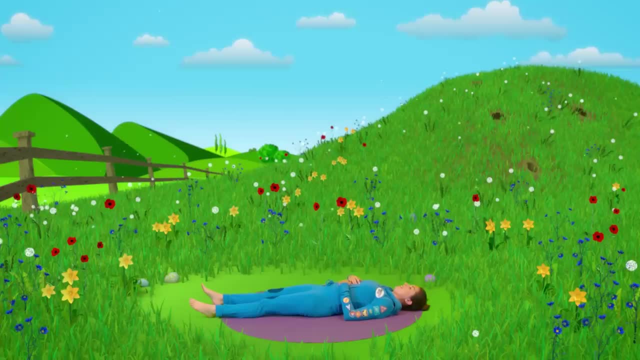 our pleases and our thank yous as well. Then everyone is happy and we know we've been good, good people. We breathe calmly and quietly here and enjoy our rest with our friend Peter Cottontail, the Easter Bunny, And then it is time for us to start to awake. 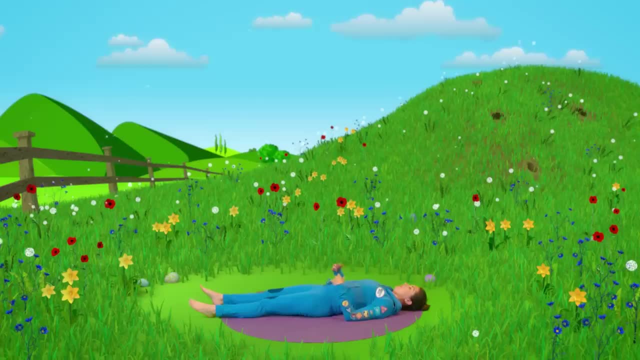 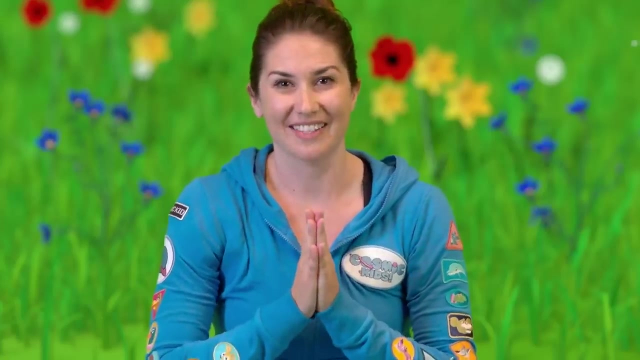 We wiggle our toes, We wiggle our fingers And we bring our knees up to our chest and give them a nice big hug. We roll over onto our sides and come up to sit with our legs crossed And we bring our hands together at our hearts. 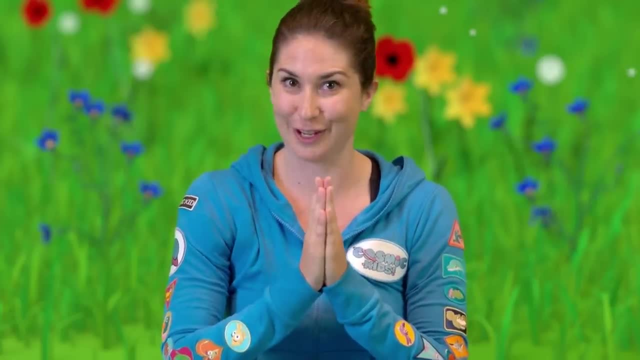 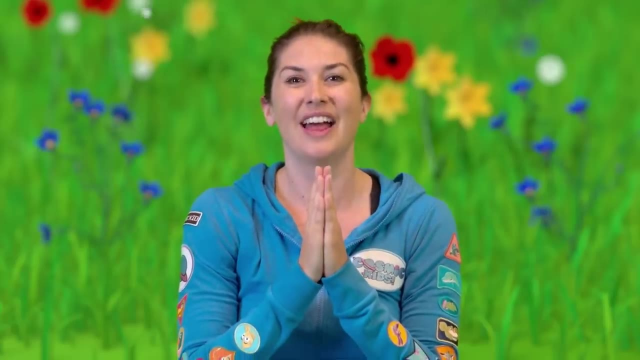 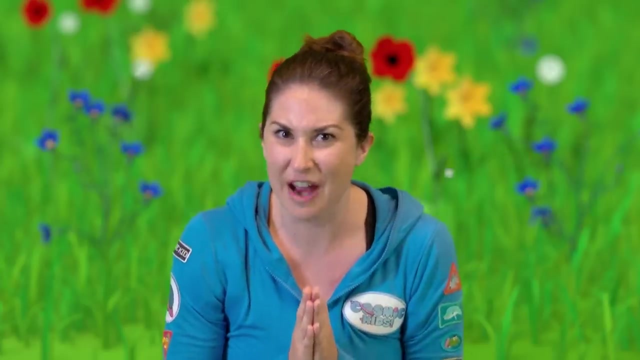 and we finish just the way we started with our secret yoga code word, which is Namaste. Ready After three. One, Two, Three, Namaste. Well done everyone. You were very brave helping Peter Cottontail rescue those eggs. 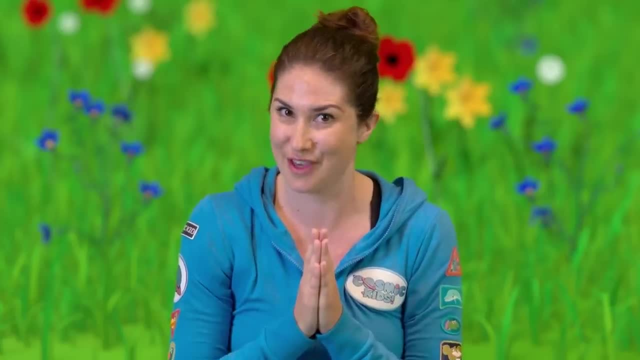 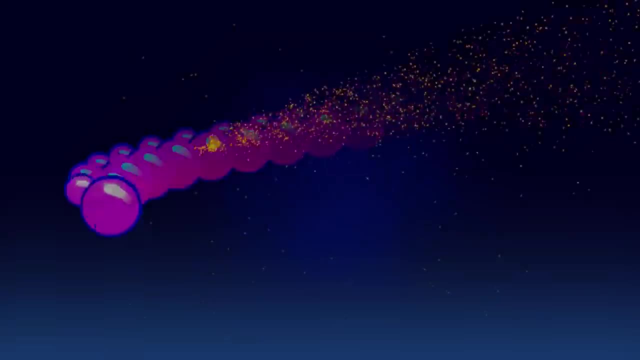 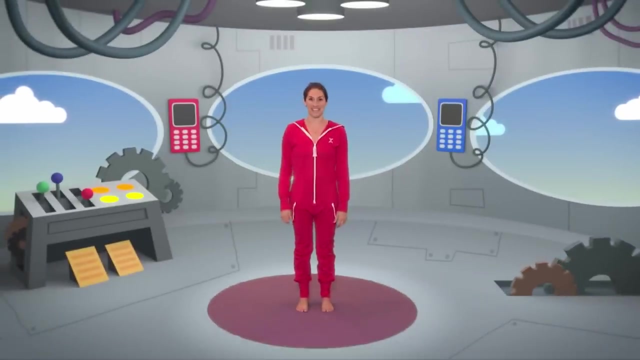 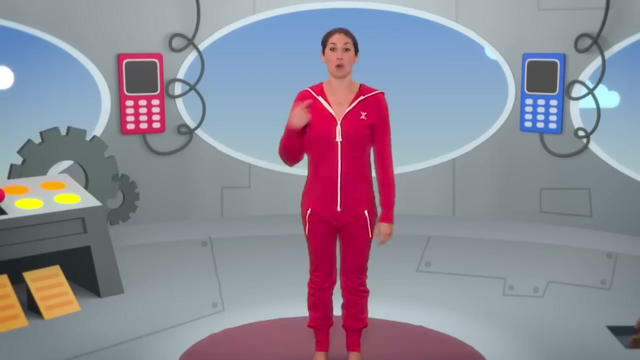 I hope you enjoyed it and I hope you come back soon for another Cosmic Kids adventure. Bye, bye, Hello everyone, Welcome to Cosmic Kids. I'm Jamie and this is your place for yoga, stories and fun. It's easy: Just copy the moves I do and enjoy the adventure. 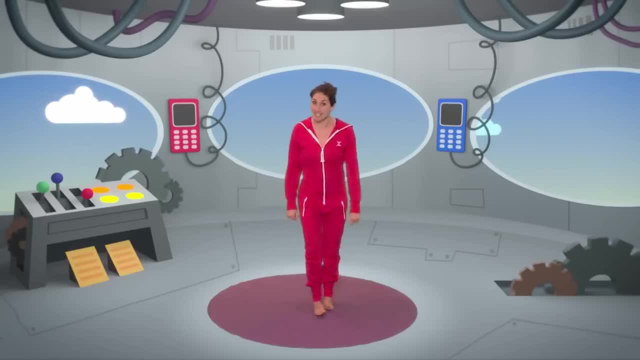 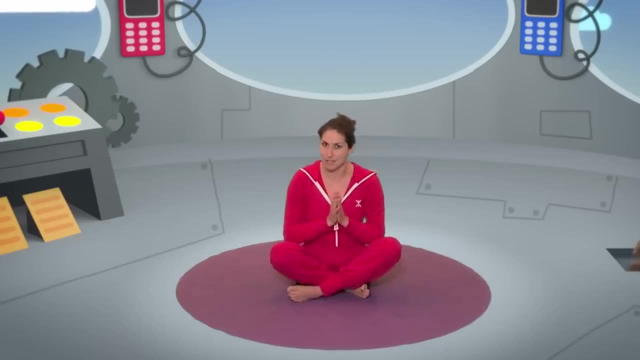 Now, we always begin in the same way, and that's by sitting on our bottoms with our legs crossed, bringing our hands together at our hearts and saying our secret yoga code word which is Namaste Ready After three. One, Two, Three. 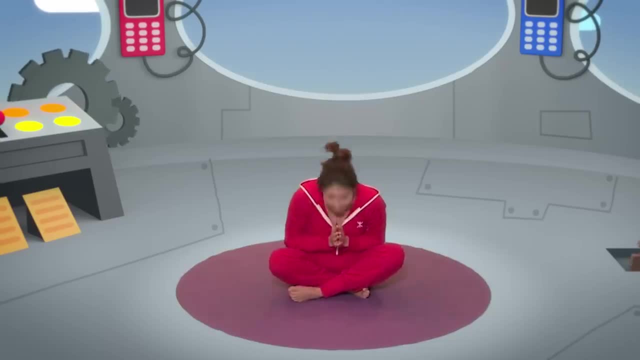 Namaste. There. Now we're ready to begin, And today we're off to meet Mike the monkey. But no ordinary monkey, Oh no. Mike is a space monkey, An astro chimp. So we're going in a rocket to space. 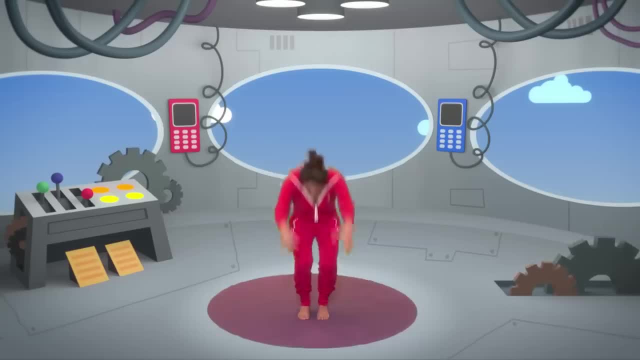 Let's go and meet him. We take the train, standing up, putting our arms down by our sides, We pull the horn, Hoo Hoo, Clickety clack, Clickety clack. Here we go Around the track. 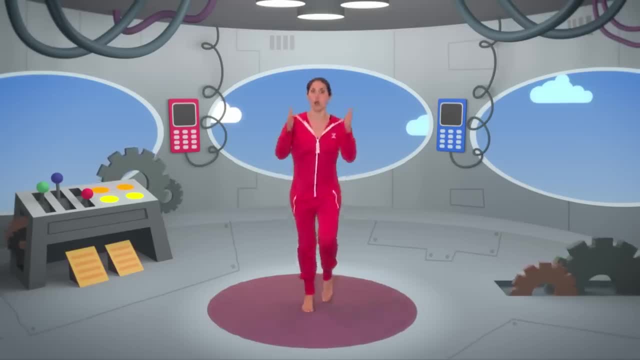 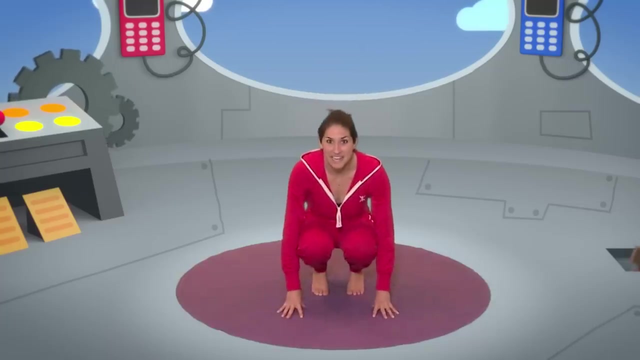 Faster and faster and faster we go, Until we're going very slow. Pull the horn. Hoo Hoo, We're here And Mike does a big monkey jump to welcome us Crouching down. After three, One, Two. 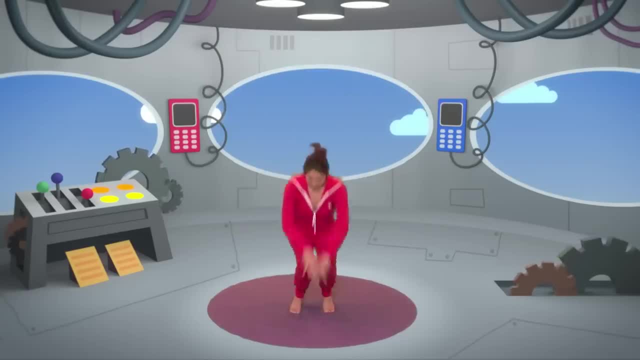 Three, Woo, Ha, ha, ha ha. He opens his monkey arms wide And gives us a big cuddle. Ooh, He leads us down through the secret tunnel, Hands down, Feet down Into the secret bunker. We sit on our bottoms. 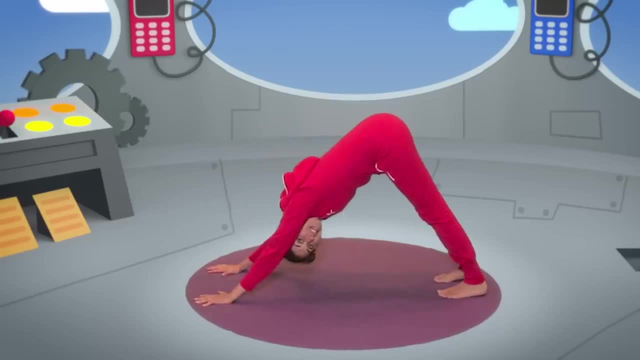 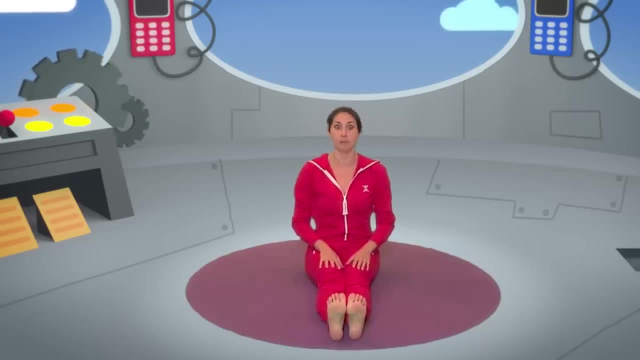 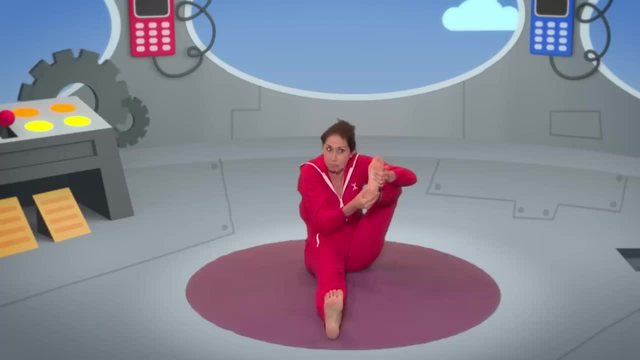 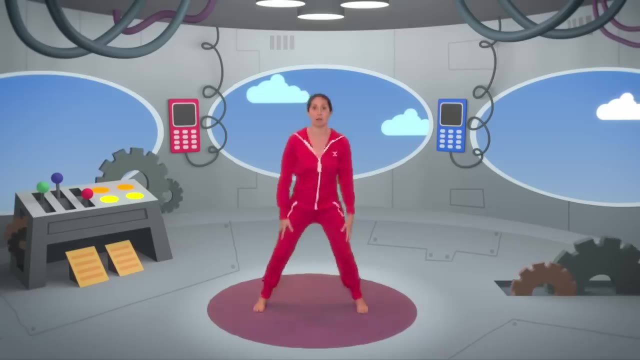 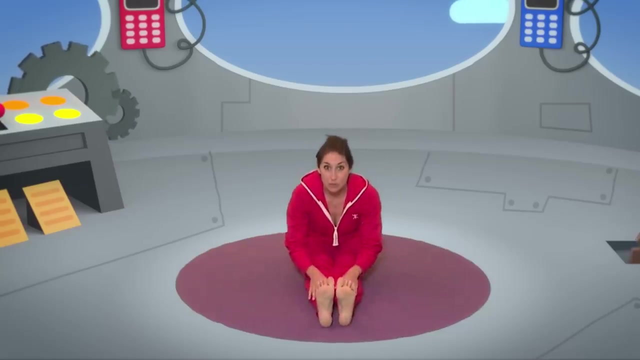 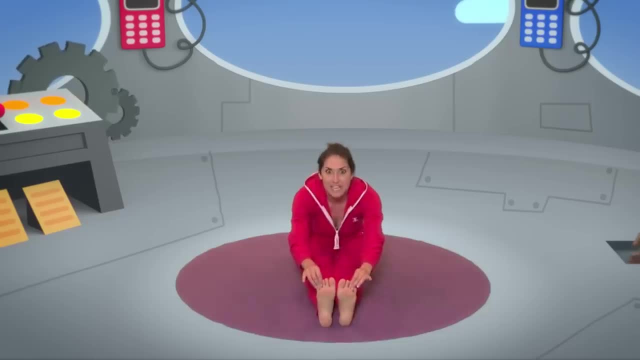 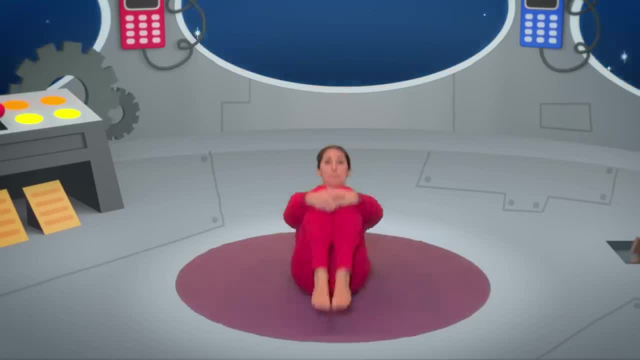 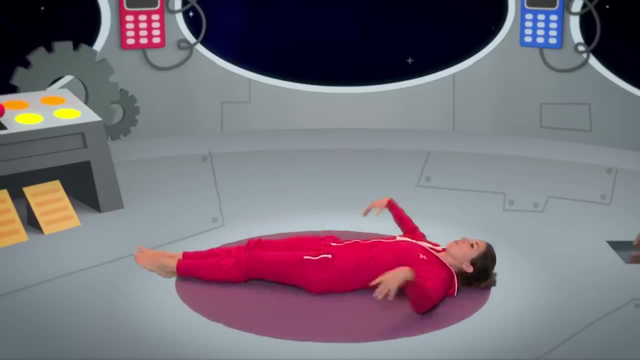 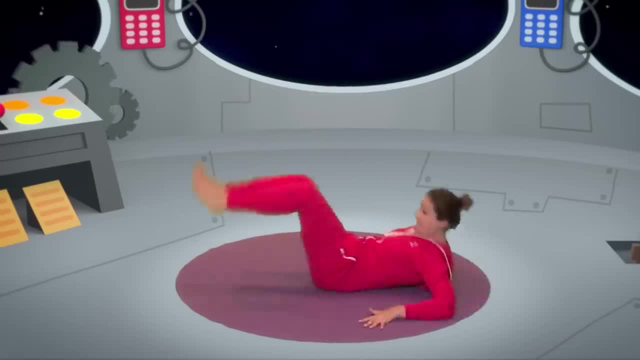 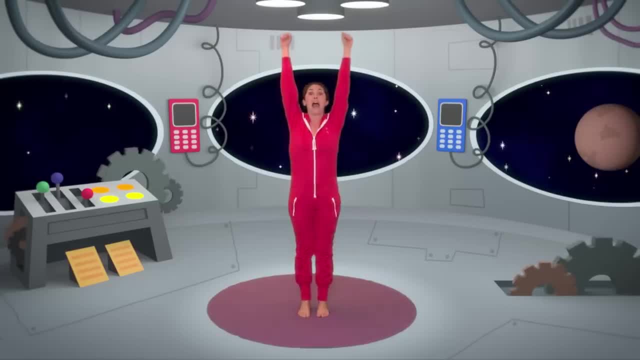 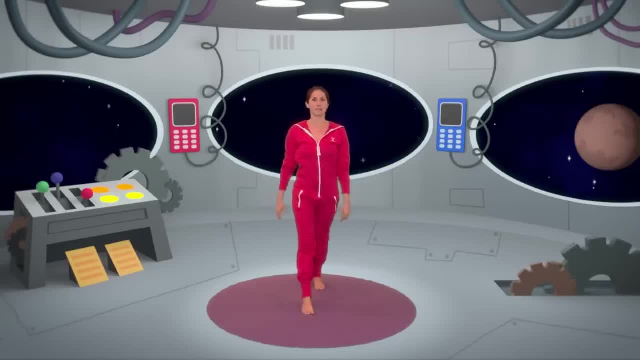 wiggle. Then he takes one small step for monkeys and looks over one side. One giant step for monkey kind, And looks over the other side. All of a sudden a door opens and out comes Mutnick, the Russian Astro Dog, Hands down, feet down, lift up your bottoms and let's. 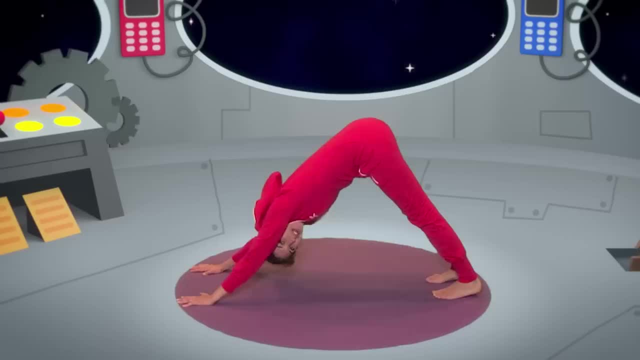 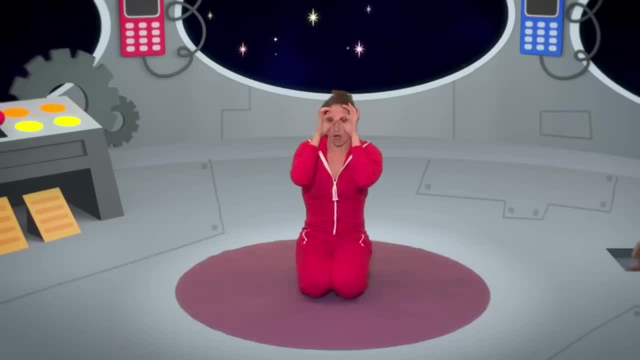 thumbs and fingers together. have a look through. There's Snarge. He's got his eyes open, He's got his eyes closed, So he's got a combined brain, really. and he's got a shell in his mud bowl Coming onto your tummy. Flick your feet towards your bottom, Take hold of your. 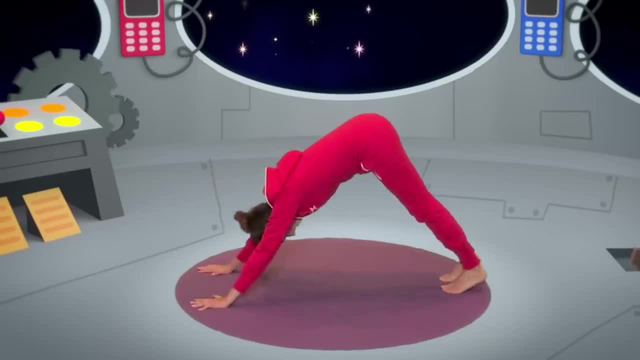 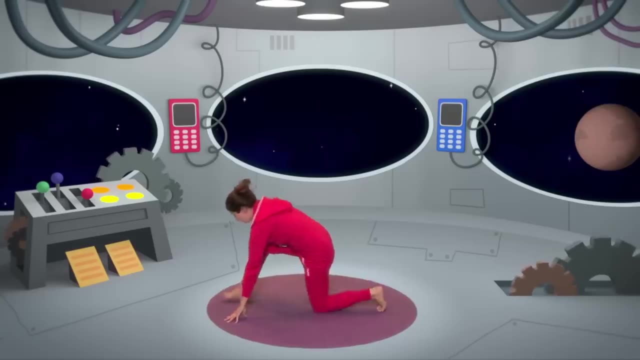 ankles and kick up like a bowl. Mutnick, donkey kicks two hoverboards free. Hands down, lift your bottom up and donkey, kick your feet. The hoverboards are a bit like skateboards, only without the wheels. They put one foot forward, one foot back and cartwheel their 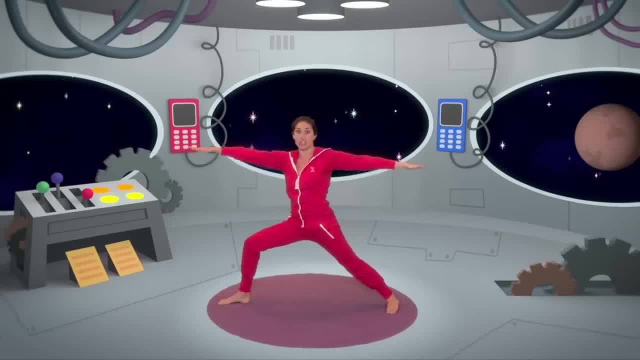 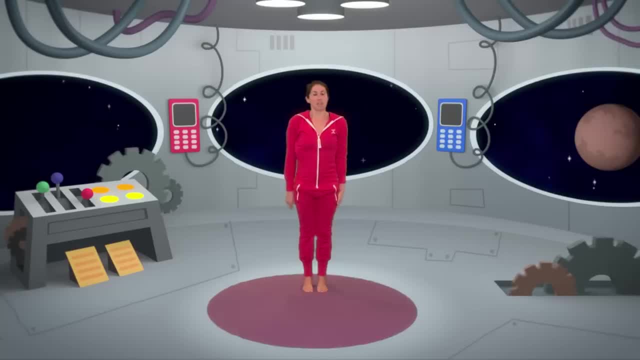 mud bowl. They're a bit nervous so they take a deep breath, criss-cross your fingers underneath your chin, big breath in, big breath out. Then they take a big squelchy step into the mud, squelch, And another big squelchy step, squelch. 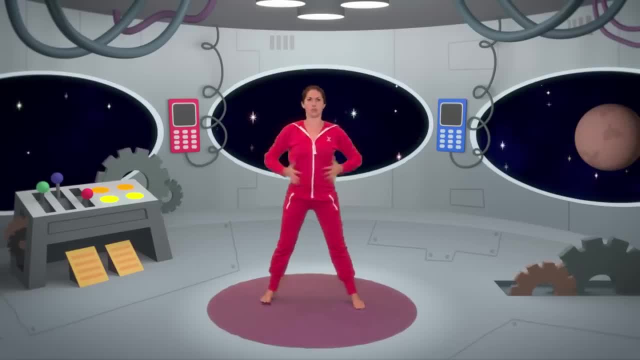 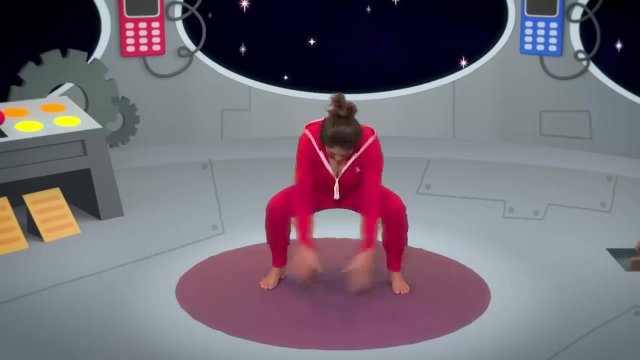 Snarge, the evil alien mudfish hears them. He says: good evening, Mr Mike and Mr Mutnick, come to save your friends. Oh dear, trapped in a cage is Gladys the spider. Bend your knees, Ticker, ticker, ticker, ticker, ticker your hands round to the outside. and Toby the turtle. 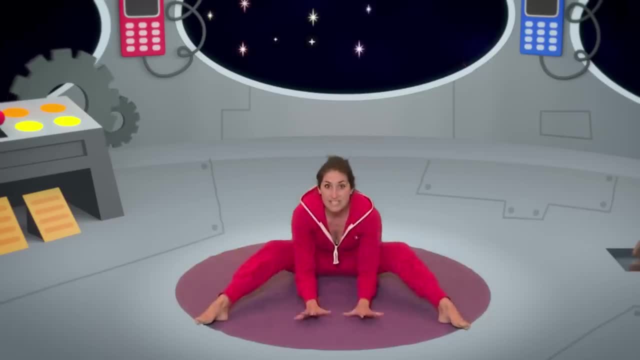 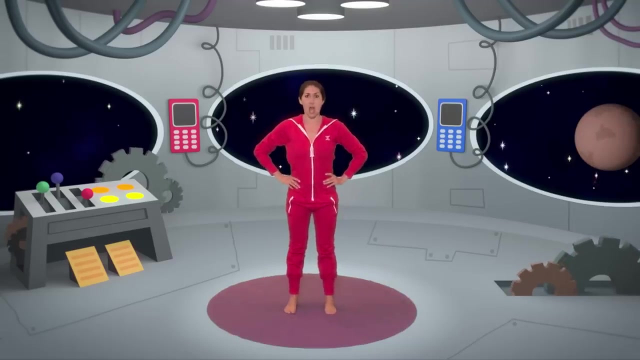 sitting on your bottom, take your legs out, wide arms inside, and under they go. Both Gladys and Toby look absolutely petrified and Mike can't bear to see them looking so scared. He stands up tall and brave and says: please, Snarge, see how they fear you. you must let. 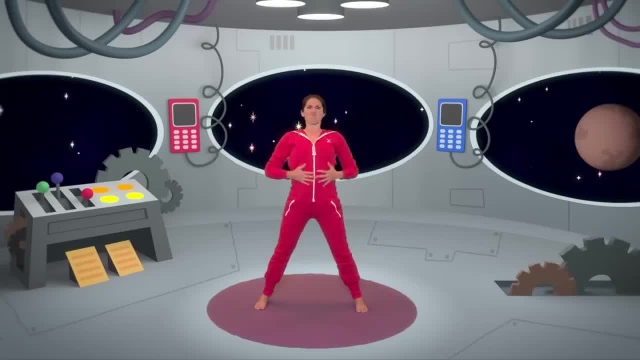 them go. Snarge jumps wide and says I don't care what they feel or what you feel, I only care about me and my feelings. But all of a sudden the whole place is hit by a cosmic storm. Millions of mini-meteors start rattling against the sides of the station and the whole place. 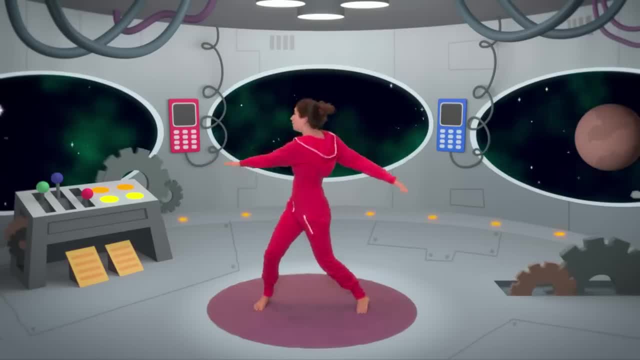 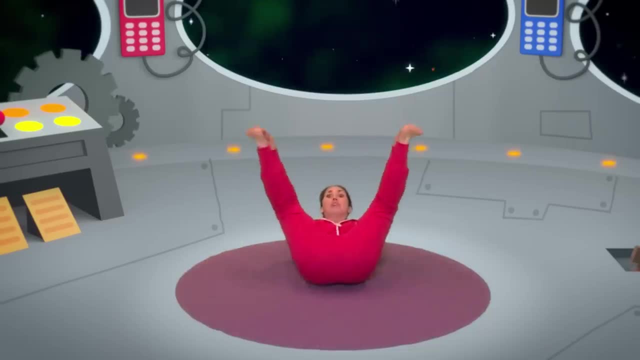 begins to spin around in a circle. They haven't got long, they've got to get out. Snarge has rolled over onto his back And he's holding onto his funny feet crying for help, Help. He looks like a great big baby. 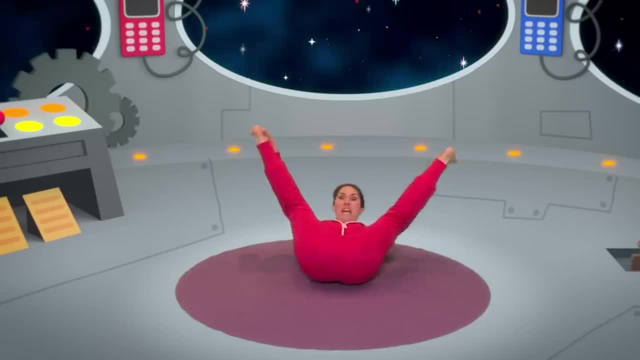 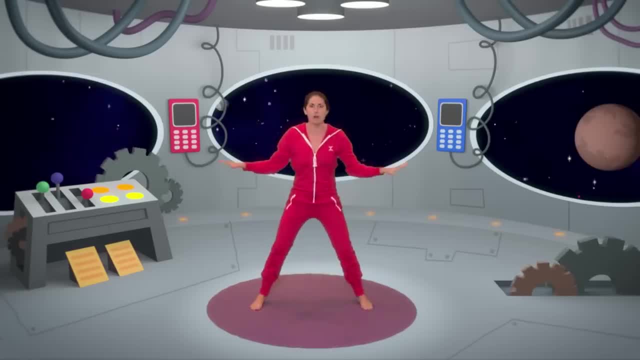 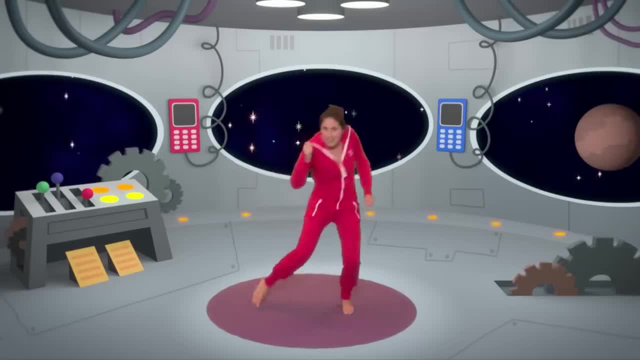 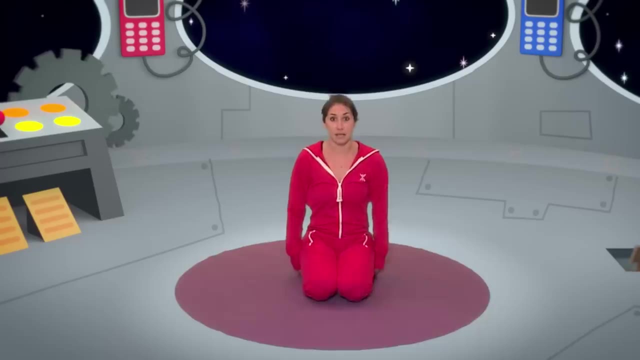 going to go back and save him And he runs In slow motion Back to save Snarge. Snarge is in a puddle on the floor but when he looks up and he sees Mike, his eyes fill with sorrow and hope. Oh Mike, please take me with you. I'm sorry, I'll stop being an evil alien mudfish. 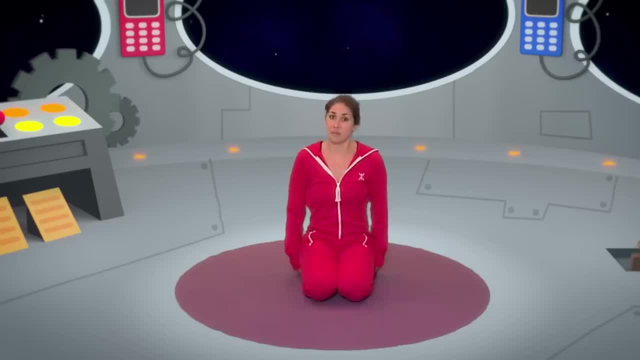 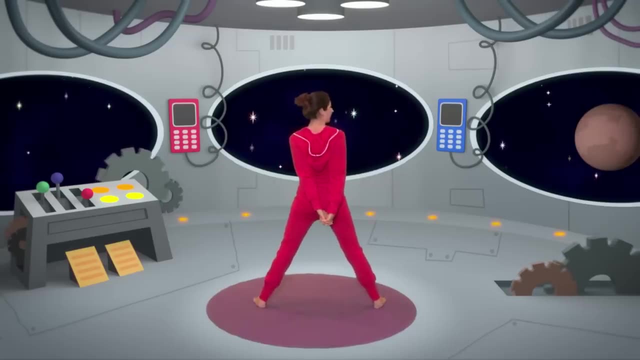 Mike knows that Snard is being real, so he saves him Standing up, turn yourself around and criss-cross your fingers behind your back. He lifts up the evil alien mudfish onto his very strong back and he clumps through the mud: Clump, clump, clump, clump all the way. 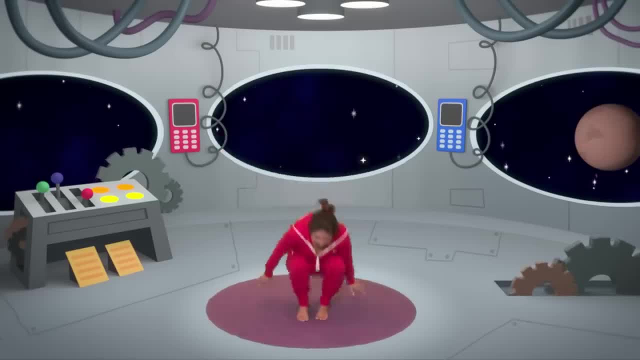 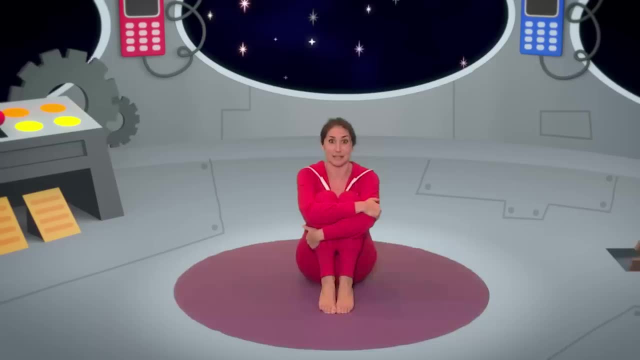 back to the escape pod. They all huddle together in a little scary huddle as they zoom back to the space base. When they arrive, Mike is greeted with a huge cheer. Yay, Everyone is delighted He saved Gladys and Toby. 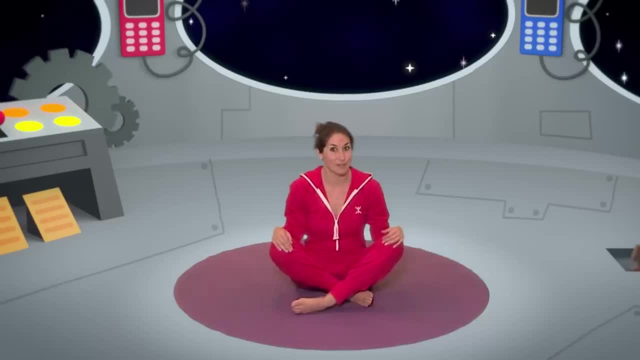 Mike is so happy. He's so ready for a rest. He takes himself to his favourite spot in the whole space base: A gorgeous comfy couch where he lays himself down, puts his arms down, puts his head back and just stops for a moment, taking some peace and quiet. Oh, what a mission. He's so pleased. 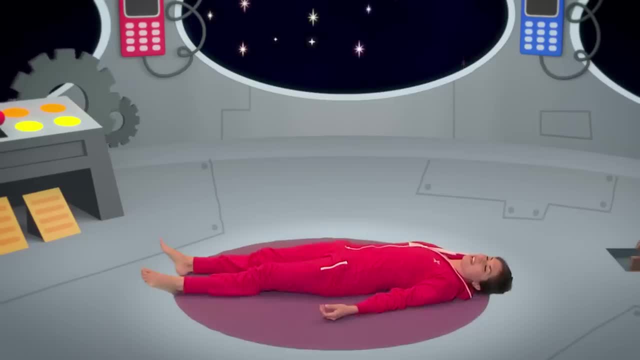 he was there to help And how he learnt to forgive someone who was clearly so bad, so pained, but needed a bit of friendship. Sometimes we have to think what other people are feeling. We can't just think about what our own feelings are And it's nice just to breathe and have some peace. 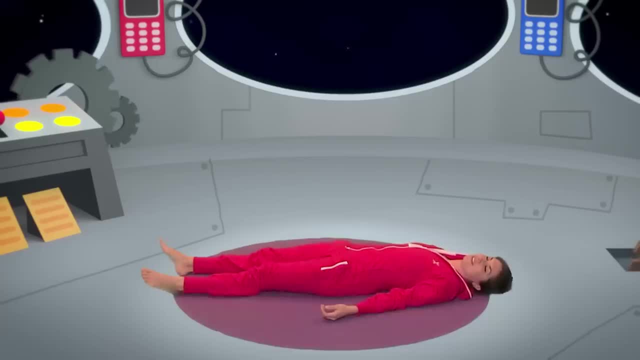 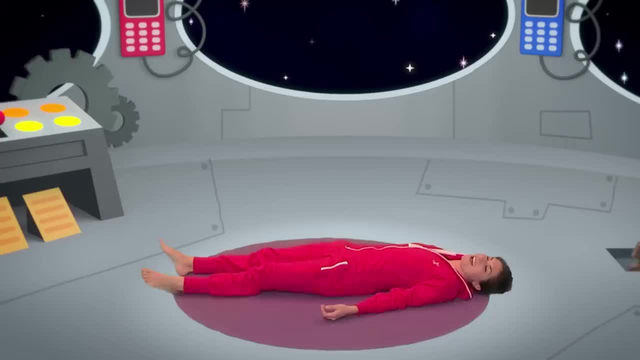 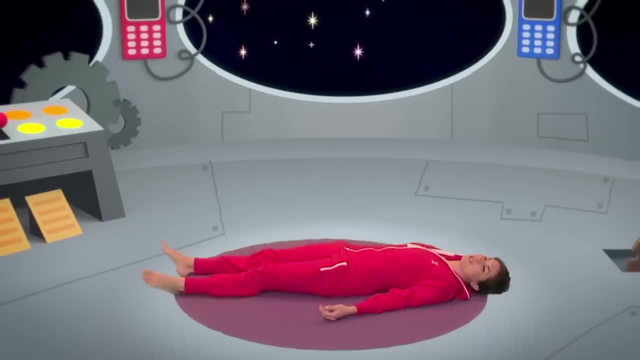 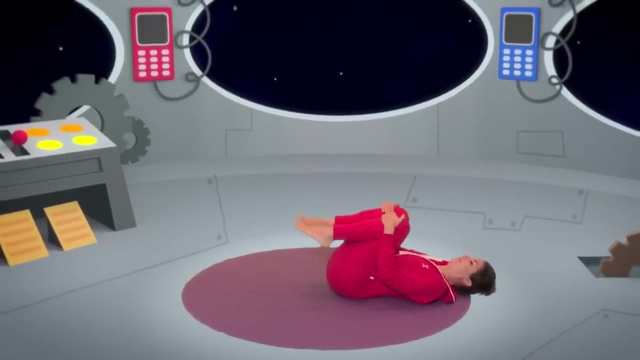 But now he feels so, pentru Now, keeping all that peace inside. slowly start to wiggle your fingers and wiggle your toes. Bring your knees up to your chest and give them a little cuddle. roll over onto your side and slowly come up to sitting with your legs crossed and your hands together. Do. 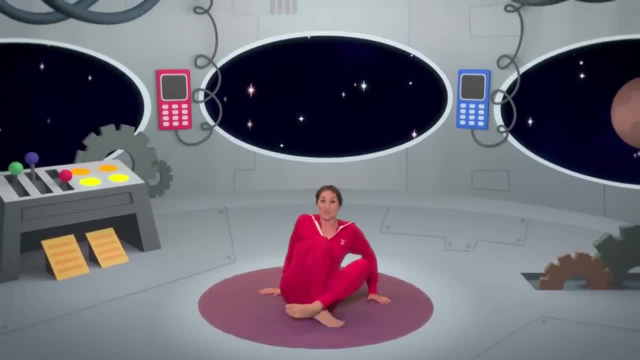 you feel your arms rolling towards your back and they're starting to feel like your arms are technically squeezing you. Now, let yourself trust so tightly and balance your muscles, connecting them to the ground, and ben dit as your head, as your nose, or with your nose persönlich, by the ear, as 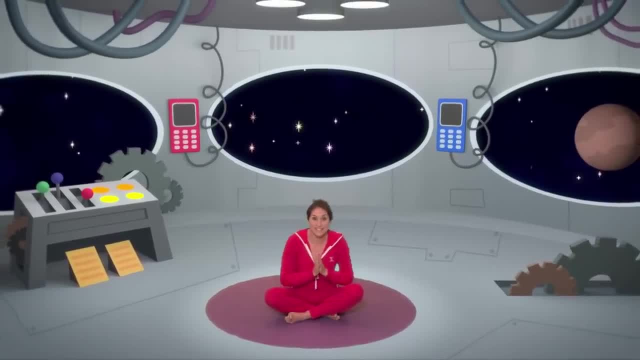 you hold your hands close to your heart as you relax immediately. Vocal compass: right your inner mountains with both legs at your heart, just the way we started. and we'll finish saying our secret magic yoga code: word: namaste, ready, one, two, three, namaste, well done everyone, thanks. 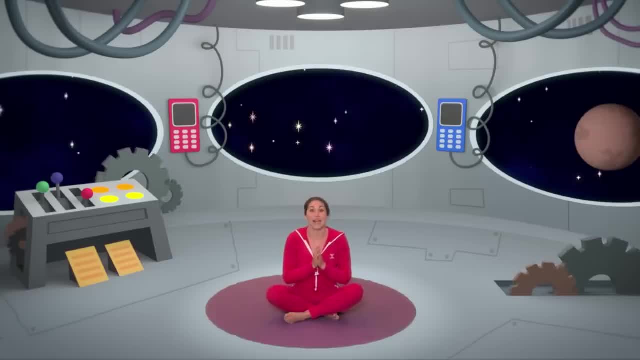 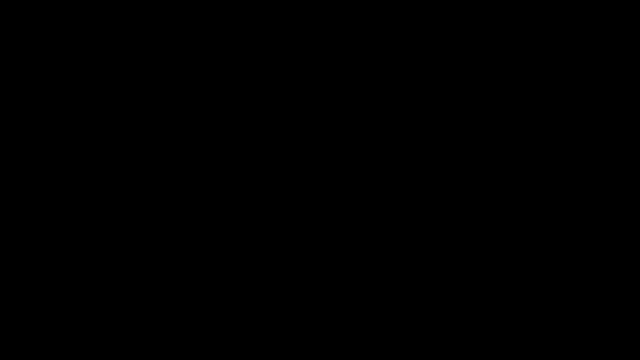 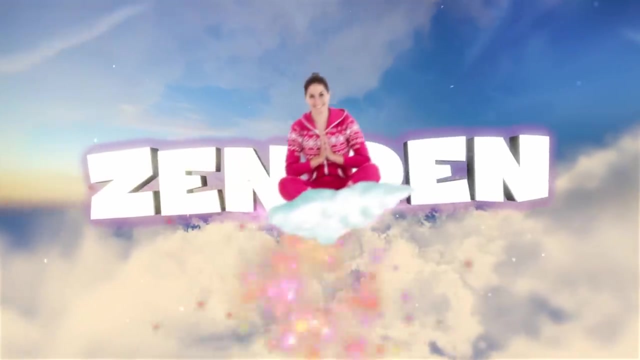 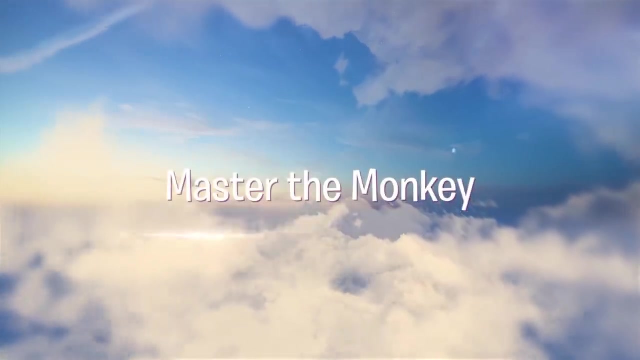 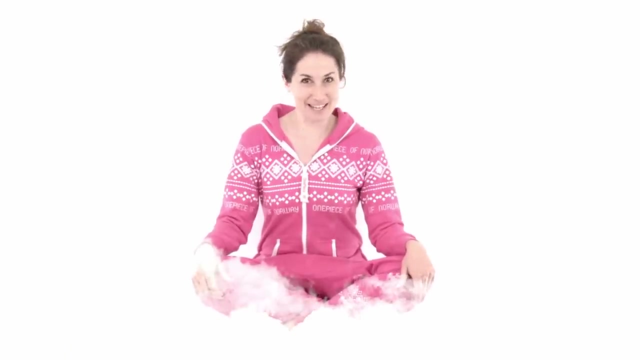 for coming to space and meeting Mike. you were great. come back soon for another Cosmic Kids adventure. bye, bye, hello everyone. welcome to the Cosmic Kids Zen Den, your place to feel calm and relaxed and to help our minds stay healthy and happy. first, let's get comfy, sit in the middle of the room and relax and relax. 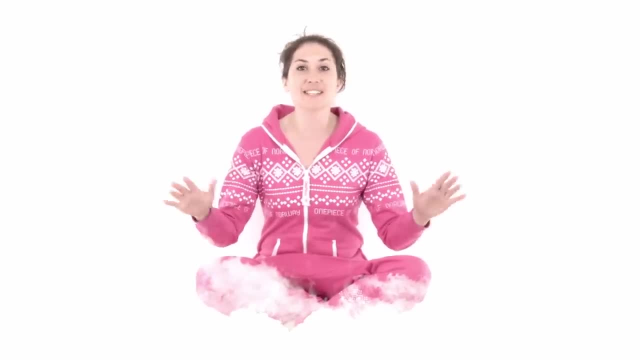 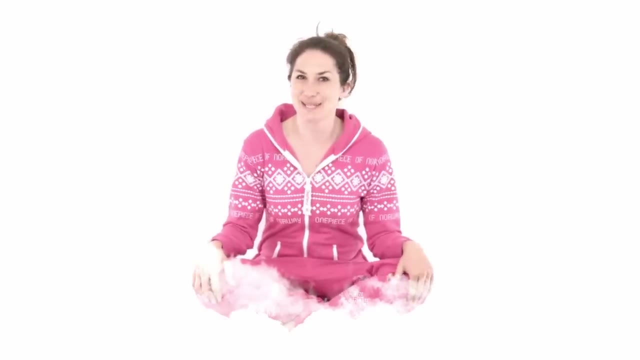 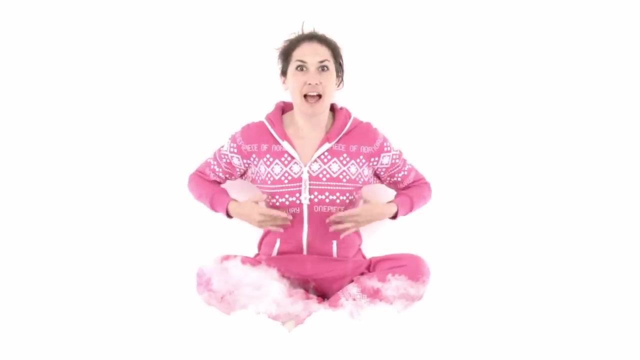 sit in the middle of the room and relax and relax. sitting on our bottoms with our legs crossed. we bring our hands to our knees and take a big, deep breath. that's better. now let's get the Zen Den ready so we can really enjoy it. we need music. let's pitter-patter our faces and bodies and 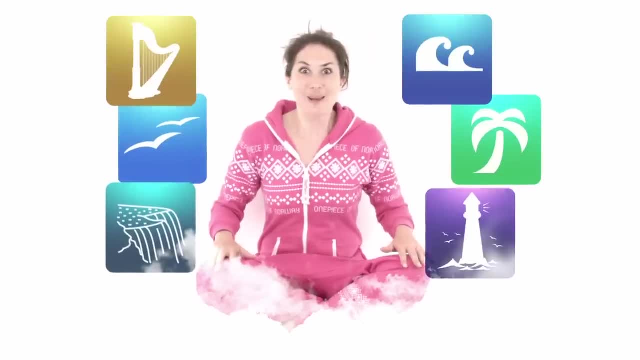 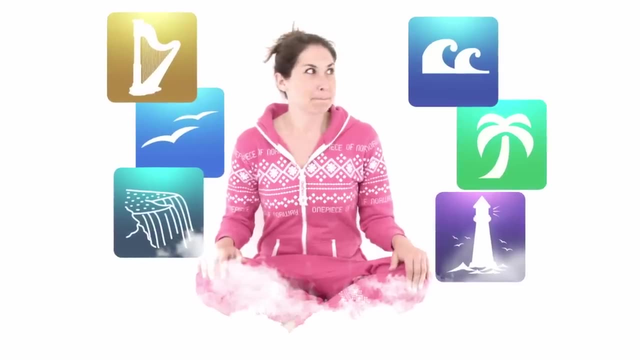 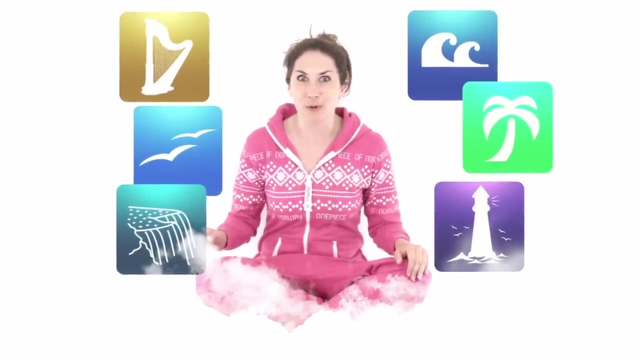 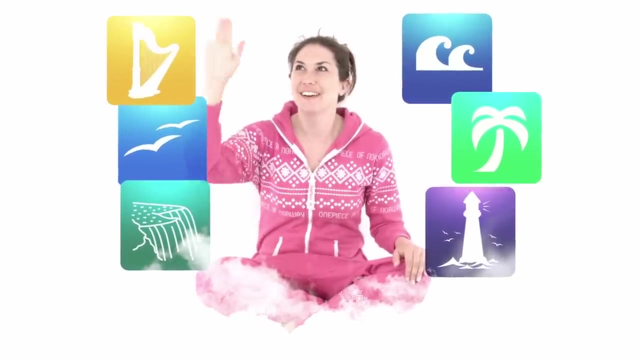 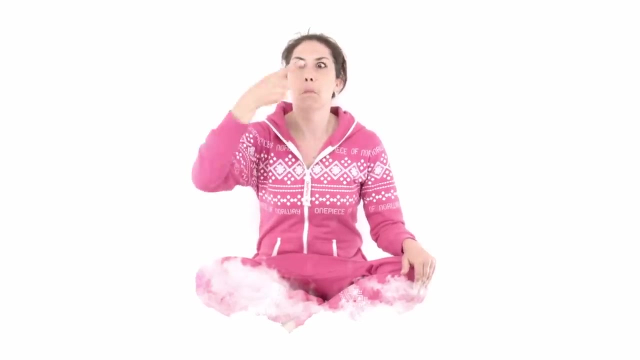 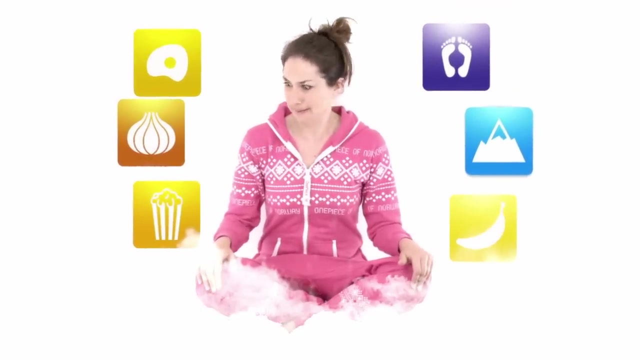 make the sounds appear. yes, well done, well done. that's it. now let's pick some that help us feel. just right: the sound of a jungle, a waterfall and a harp. perfect. now for the smell. let's press our nose button. yes, we did it. Brilliant work, everyone. Now what have we got here? Wow, the smell of feet, An eggy. 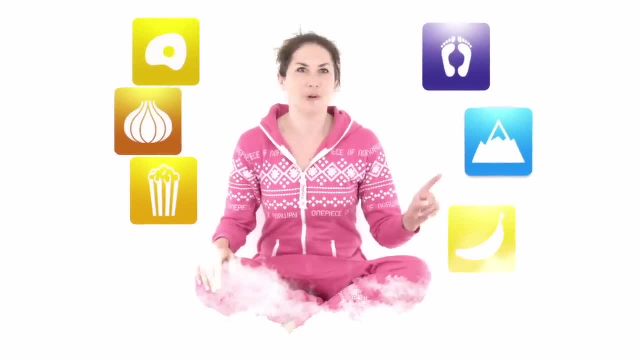 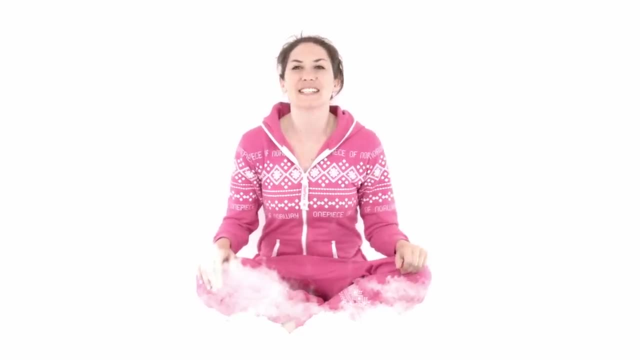 smell. Hmm, let's smell the mountain air. Yes, that's a really clean, fresh smell. We're going to play a game called Master the Monkey. You get super power points for this game. Every time you breathe in slowly and breathe out slowly, you get one point like this. That's one point. 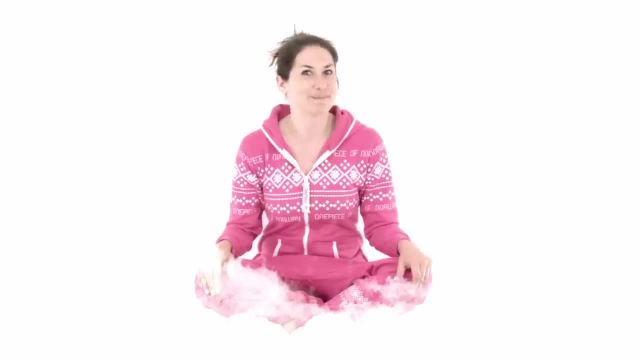 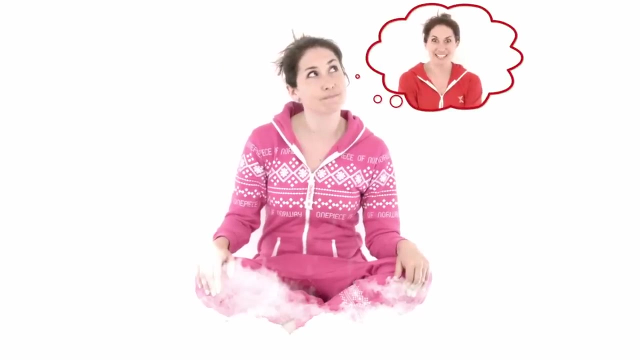 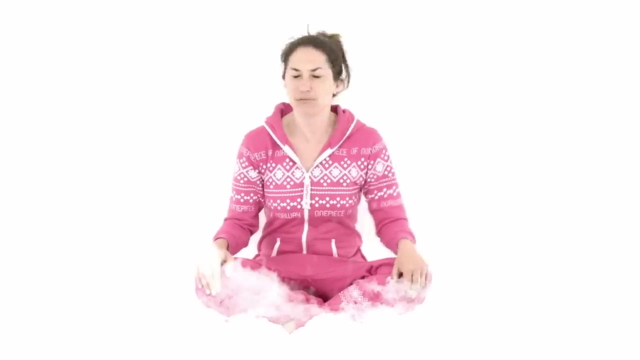 Sounds easy-peasy, yes. Well, here's the challenge. In your mind, there are lots of thoughts whizzing around stuff like I wonder what's for dinner tonight. I'm going to a birthday party on Saturday. Where did Keira get that sticker? I want a sticker. 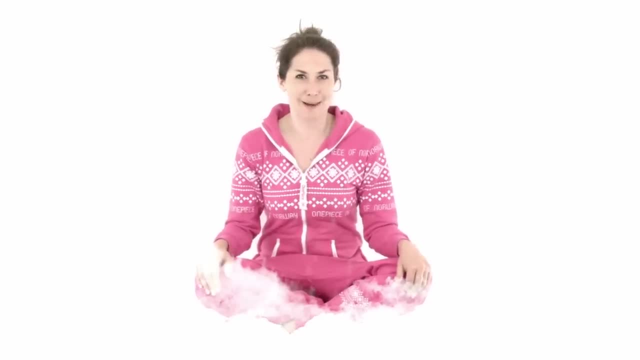 Brrr. Our mind can be a little like a monkey, sometimes jumping all over the place from one thought to the next, It never seems to stop. There's always another thought to jump onto, and another one, and another one. If we can learn how to give our monkey mind a rest for a while, 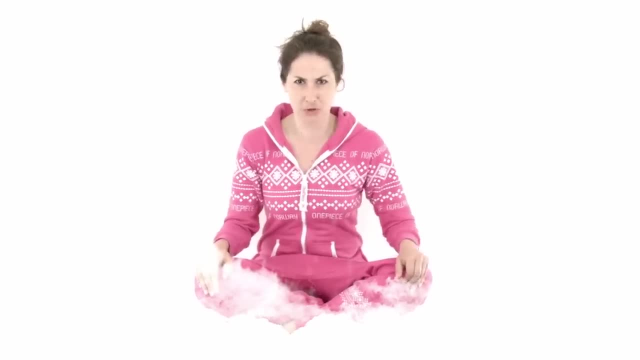 we get this superpower called concentration. To get this superpower concentration, we need to collect superpower points. Remember the breaths. For every breath you do in and out slowly, you get one point. See how many points you can get.